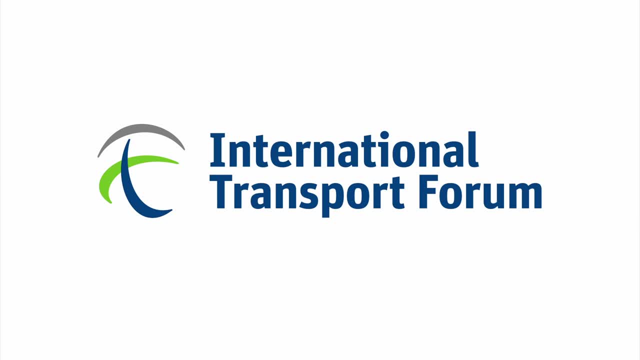 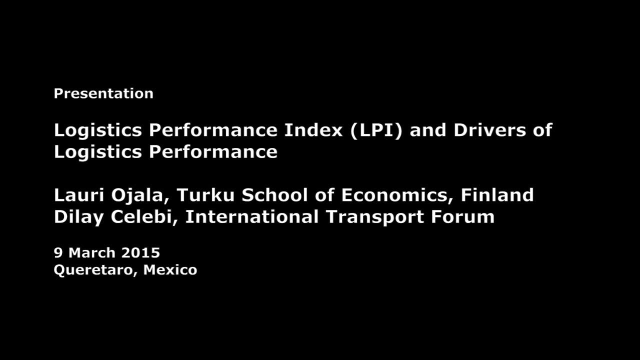 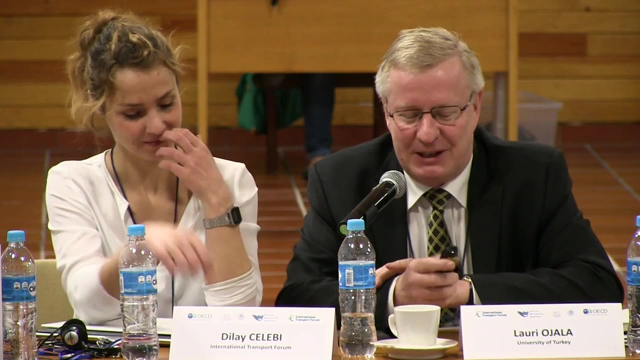 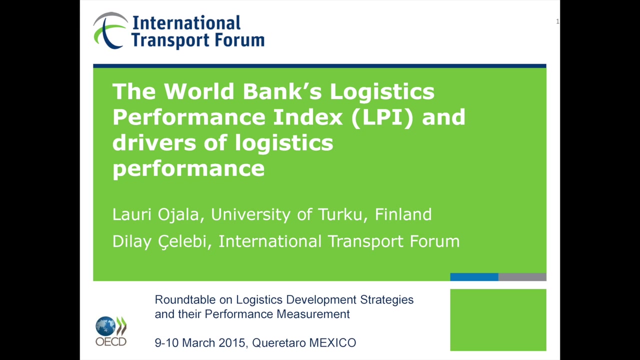 First of all, we start with a quick slice on Turkey. some of the background, because this is about a case study applying the findings from the World Bank Logistics Performance Index- broad indicators- to Turkey and to understand better what does this LPI actually? 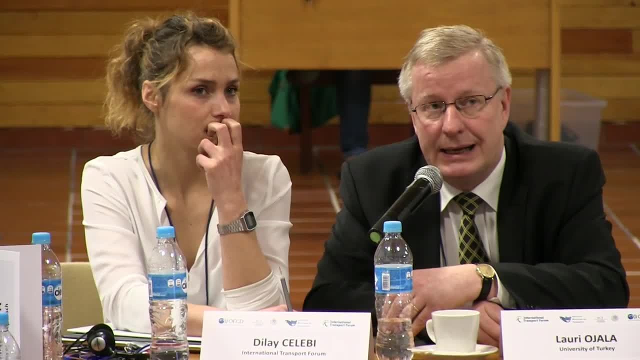 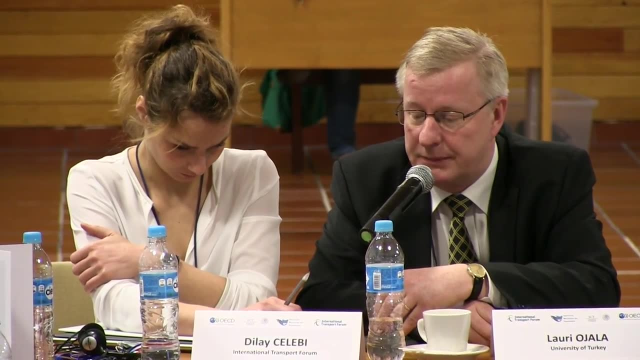 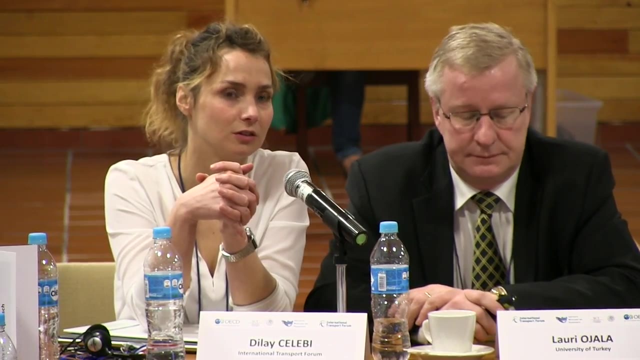 tell and to look further in detail inside the country. how well does it fit the actual situation on the ground? But maybe, Dilan, you will say a few words about Turkey first. Thank you, Larry. Yes, for the ones who don't know where Turkey is, well, it is located in between more or 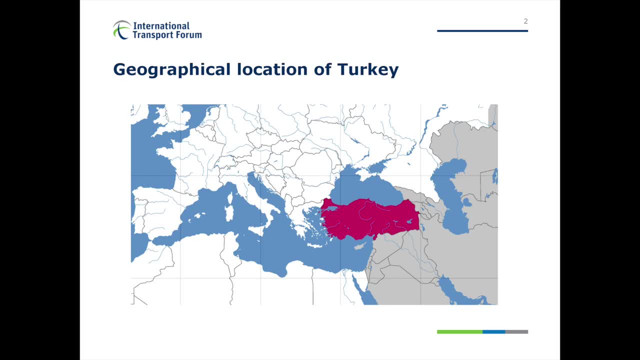 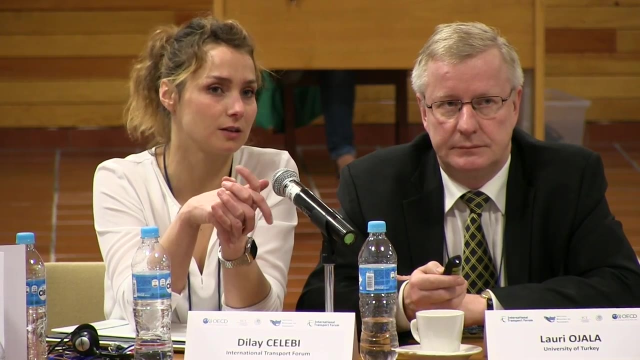 less you could say Asia, Europe and Africa. so it's geographically very much suitable for such a case study, for being in between the major transportation roads or just lines, And also it's an upper-middle-income country with a growing GDP. 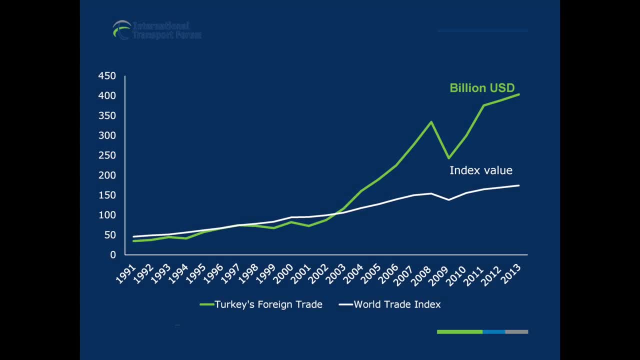 So with the increasing foreign trade, you can see that in the last couple of ten years, after mainly just a mere point here- here you see the agreement with the European Customs Union, with the European Union, the foreign trade has increased tremendously, almost five. 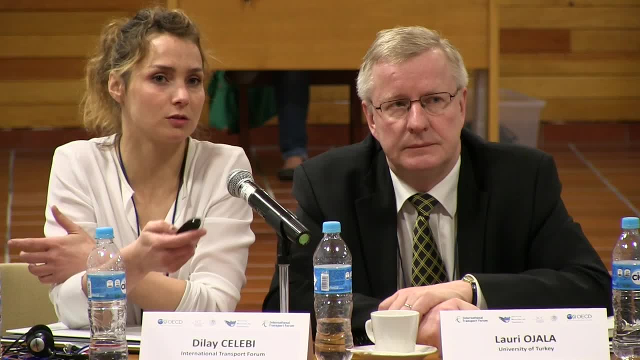 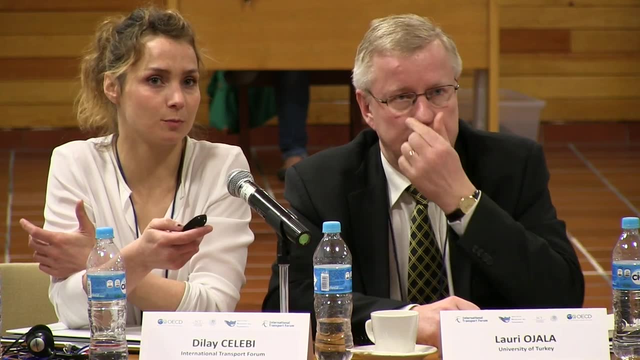 times just in the last couple of ten years. So it's also. So it's a good case study for us because we are investigating the logistics performance index and since it's a kind of a statistical measure, maybe Larry can explain you better. 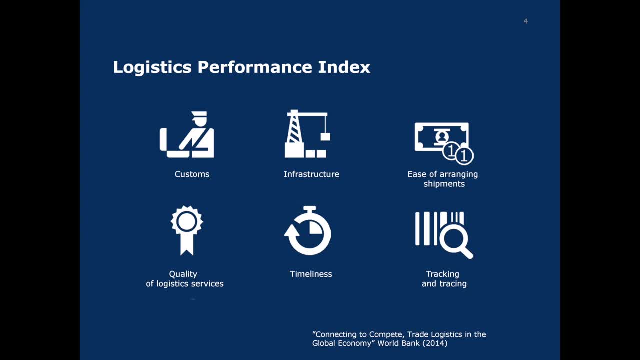 later that the confidence intervals of this measure for Turkey's performance is quite small. so which gives us more reliable just data on logistics performance. Very good, Very good. And now that we are here in Mexico: Mexico has a population of about 120 million people. 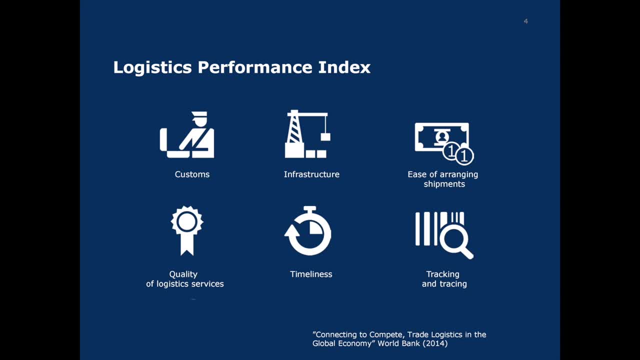 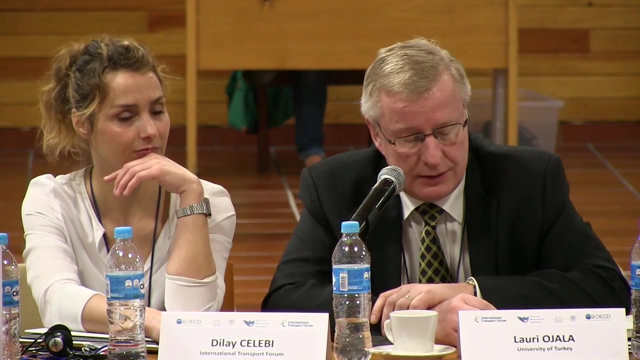 Turkey has close to 80 million people, so there are also in that sense a few resemblances as similar type of order of magnitude of countries in that sense. So what we have done here was actually initiated by the Turkish government partly and done. 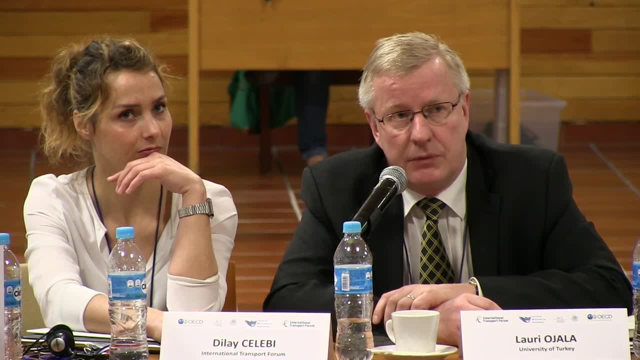 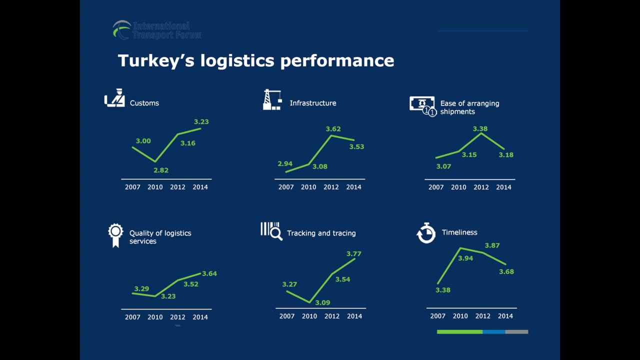 under the auspices of International Transport Forum And also for international transport. Yes, In the last nine, ten months we spent a couple of weeks or two weeks in And Delay. of course she comes from Turkey and knows the country, but we spent some time. 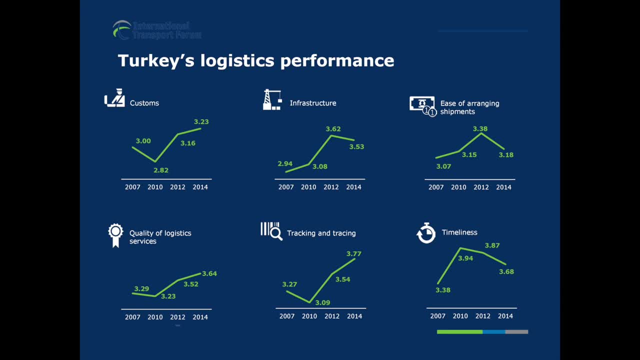 in having extensive interviews with stakeholders in Turkey, looking at those broad areas, that also the logistics performance index is covering mainly the customs and border agencies, meaning that how easy or difficult it is to organize trade logistics to and from What is the level of? 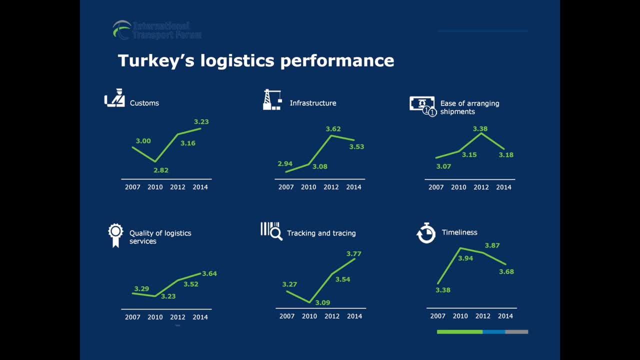 Excuse me, Level of transport and also telecommunications infrastructure and services in the country used for transport and trade and logistics. how easy or difficult it is to arrange shipments to and from countries. meaning capacity, affordable capacity to and from the country, Not looking at specific modes in this LPI international comparison. 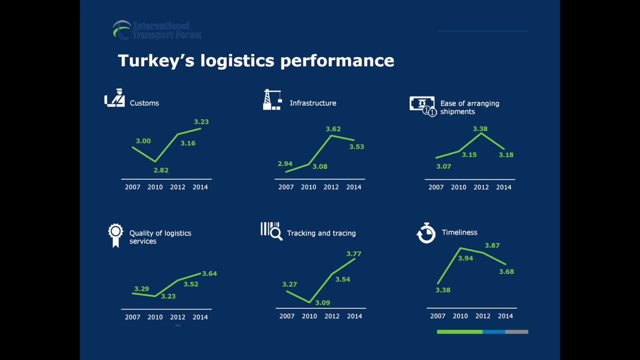 We did not have questions In this index. We do not have questions on how would you rate the road transport. how would you rate the rail transport, which is more broader based gorge Quality of logistic services you find in the country reliability issue covered by a question. 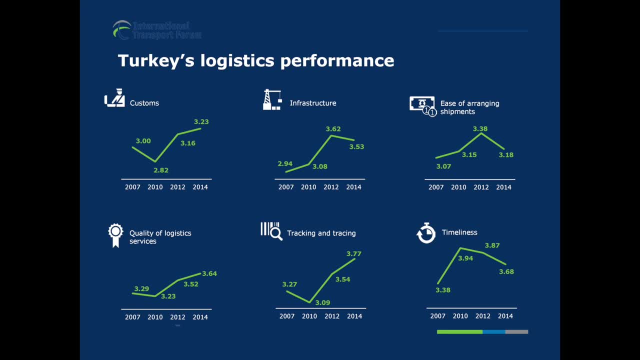 of timeliness and how easy or difficult it is to track and trace, And this is now the fourth edition of the LPI. The first one was published 2007.. And this was released. The first one was published in 2007.. 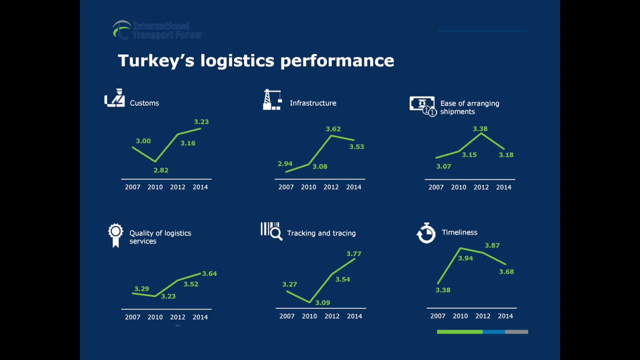 This was published almost exactly a year ago, or 11 months ago roughly. This is a worldwide survey among freight forwarding logistics people And this also means that when we address and have approached freight forwarding people, the findings are more applicable to manufactured unitized type of transport than, let's say, 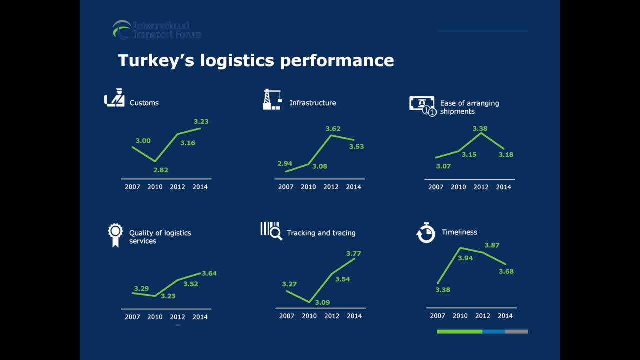 for example, bulk transport of iron ore or oil, crude oil, because there you don't usually have freight forwarding people as middlemen. You have other ship brokers or you have some closed-loop industrial arrangements, But here we have freight forwarders. it's more like a manufactured value-added, higher-value-added. 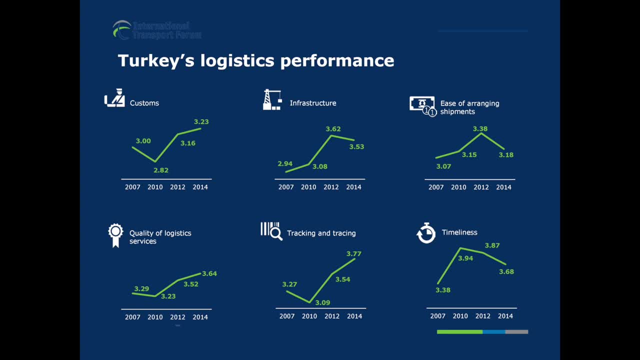 type of goods- And this is just a snapshot from this- along these four editions of the LPI: 2007,, 2010,, 12, and 14.. This just gives a quick idea of the change Of the changes. 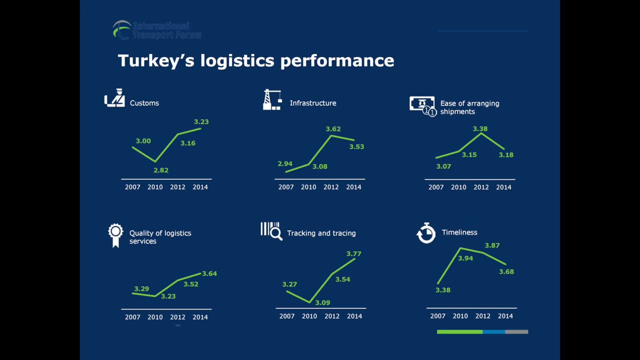 Of the changes, Of the changes, And we can see that Turkey's scores along those six dimensions- and these six dimensions are the ones we use in the international LPI, when also countries are compared to each other and their rankings are produced- Broadly speaking, you can say that Turkey, if you start from the rank, has been among: 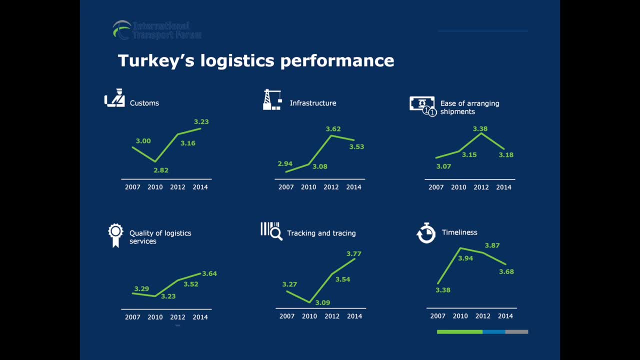 the ranked 30 out of 150 or 160 countries, most recently, I see. So it is in the top fifth, if you like, of the countries that we have measured worldwide. It has also shown quite some improvement in how customs and border agencies are performing. 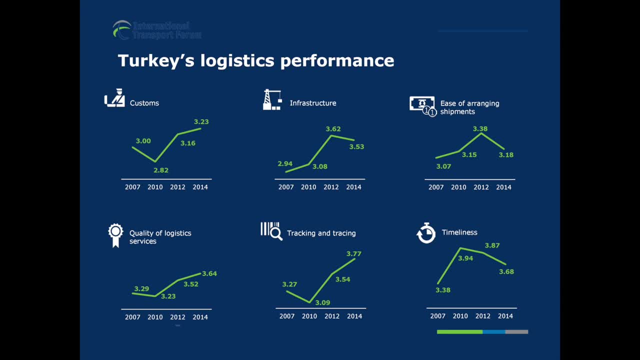 and also how easy or difficult it is to track and trace shipments, and also the quality of transport logistics services has been increasing, Generally speaking, also that of transport-related infrastructure. 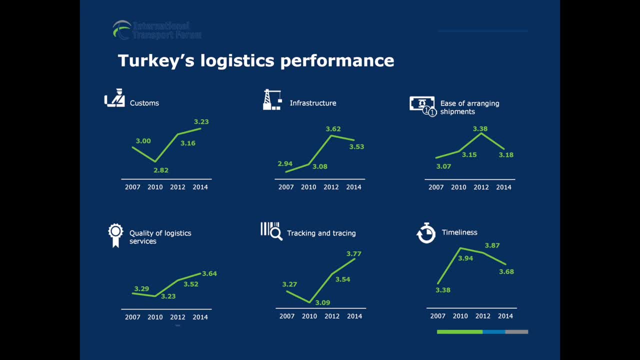 There has been some downward ratings or scores for timeliness and ease of arranging affordable shipments, But generally speaking, dessert. 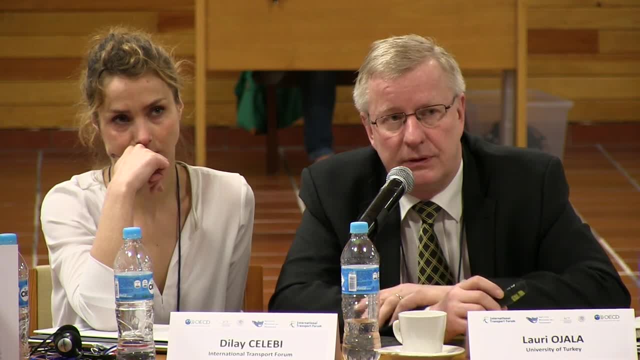 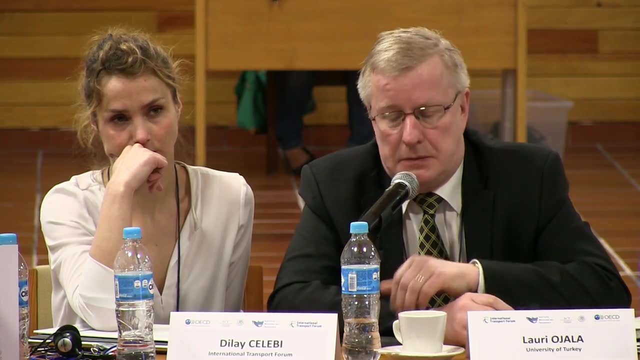 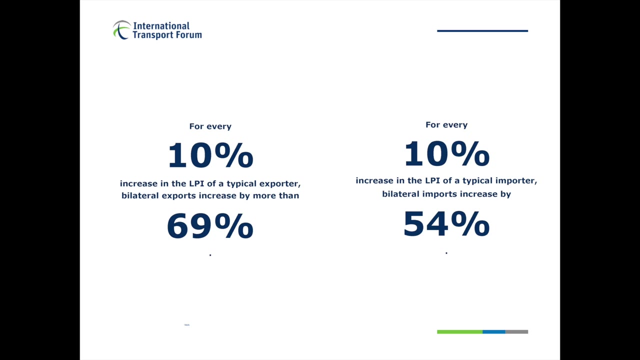 Turing out with technicianning performance in the top fifth of the countries all along, And when we look at the macro-data and compare it with the world trade data- even though this is not a porcelanity that we are advocating, but we find that each of these countries has 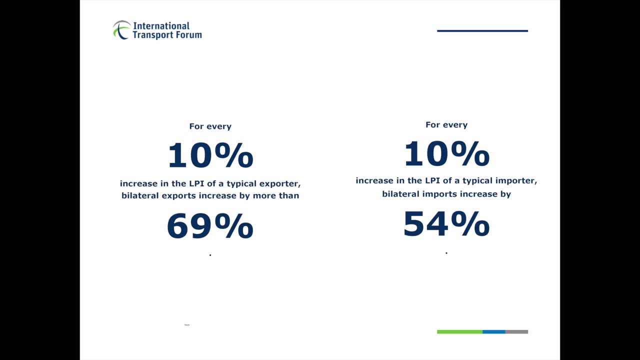 oxidised their lack. someday this shady market will become in our Ens coping that if you would take any country that could increase its logistic performance index score by 10%, not the rank. 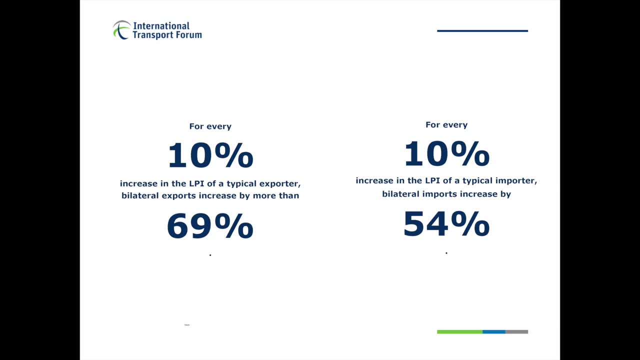 but the score by 10%. that would mean that, comparing with the World Trade data, it would correlate with a 69% of increase in exports for that country, And for every 10% increase in the LPI score for importers or imports, you have a 50% plus 54% increase. I stress this is not a causality, but there is a strong indication- as Jan was interested with some other human development index or corruption perception index- that how well and how easy countries are to organize trade logistics is significant, how much they are engaged in world trade. 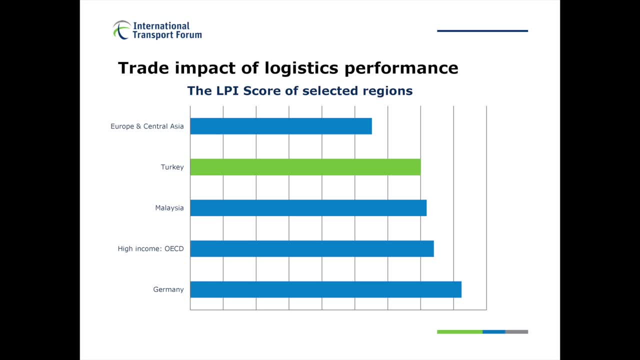 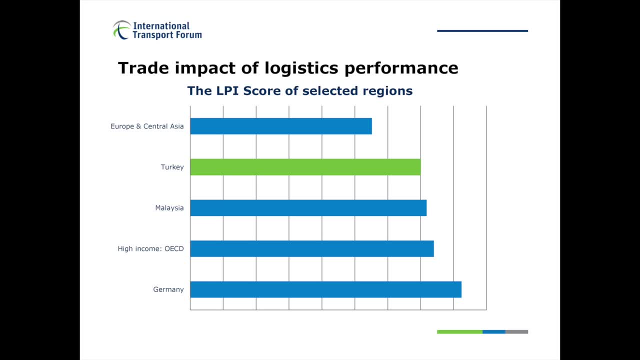 or otherwise relevant trading partners for Turkey. Malaysia was chosen as one of the competitors because it is also in the upper middle income class And actually the top in that income group, where Turkey comes second And if you take a look at the overall LPI score. 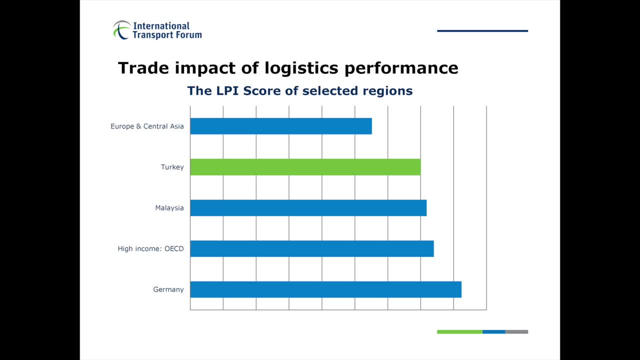 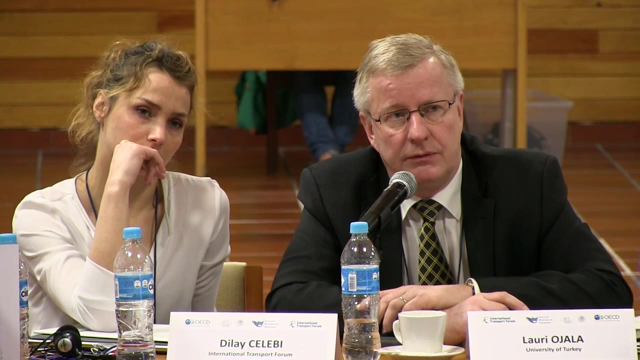 Turkey is not very far from the high income OECD average. Germany came as the number one country in the 2014 LPI. It also did so four years ago- But if you compare it with the World Bank group Europe and Central Asia, Turkey is performing clearly better. 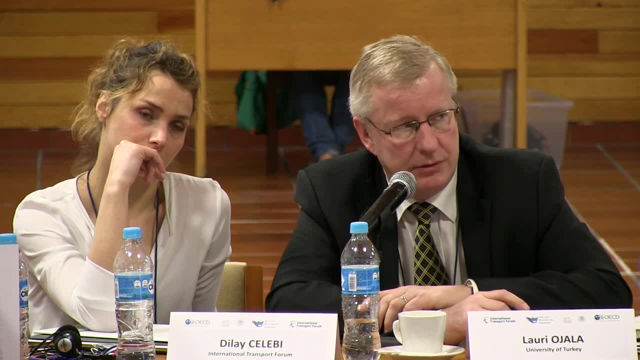 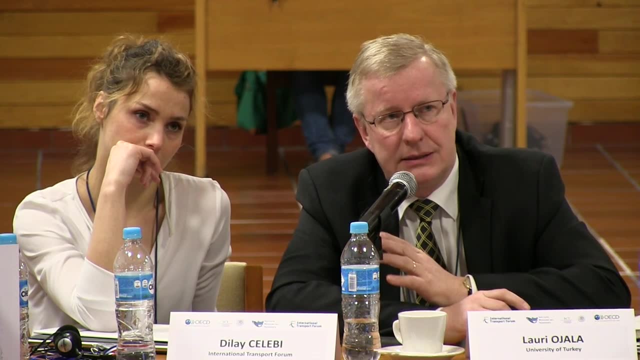 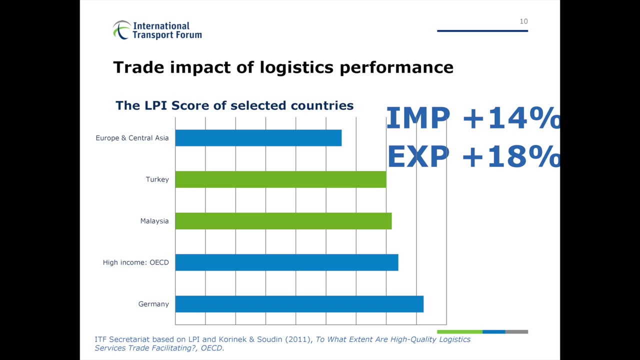 Now I have to say that Europe and Central Asia is excluding, including European Union. That's the country region which does not have European Union, but it has the non-EU countries and Central Asia as a competitor. If you look at the logistic performance index, 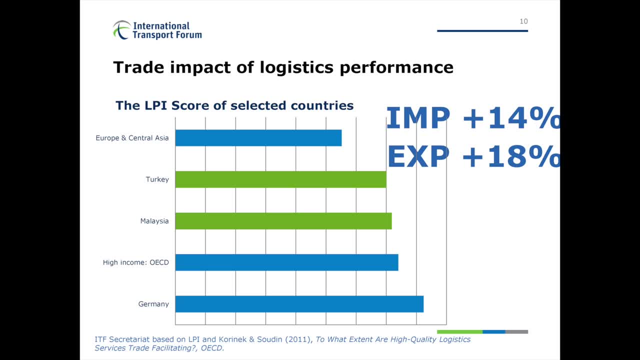 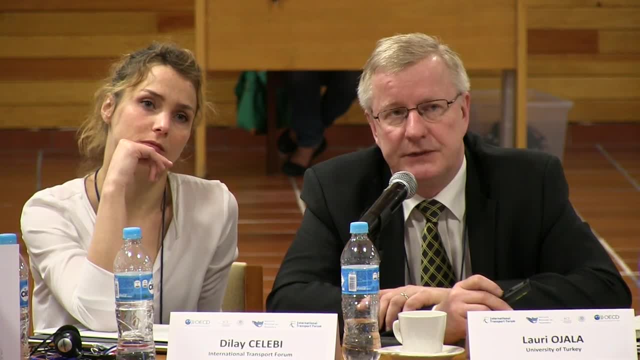 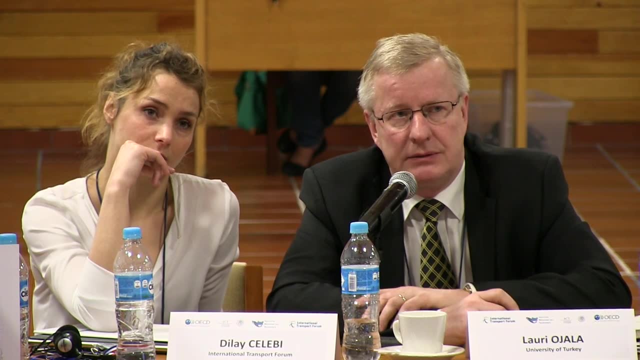 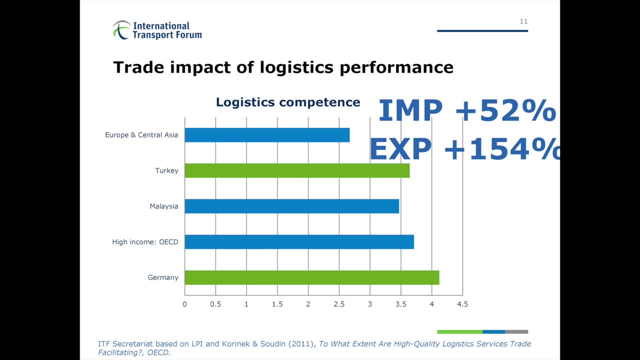 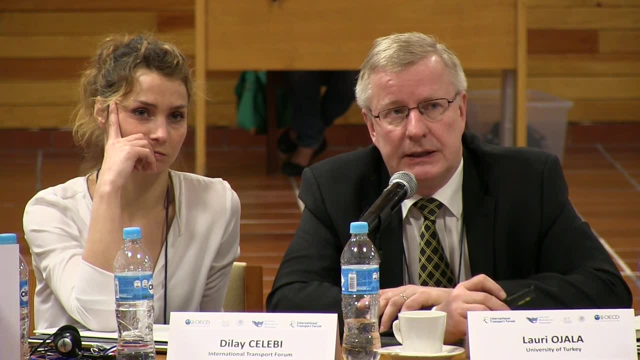 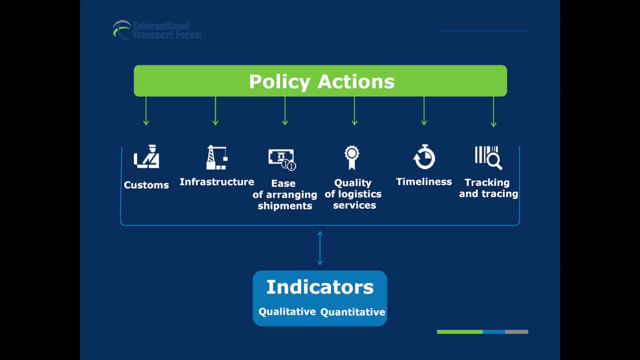 would mean a significant increase in exports, something that turkish now. the policy actions that we try to understand better, doing the field work and interviews- quite significant number of interviews with key stakeholders both in industry, trade, logistics and government, to understand how do these six dimensions in the lpi 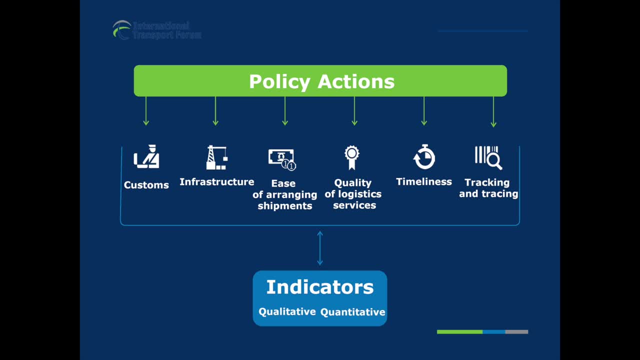 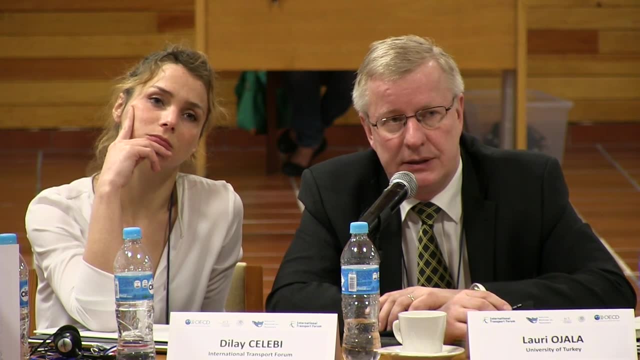 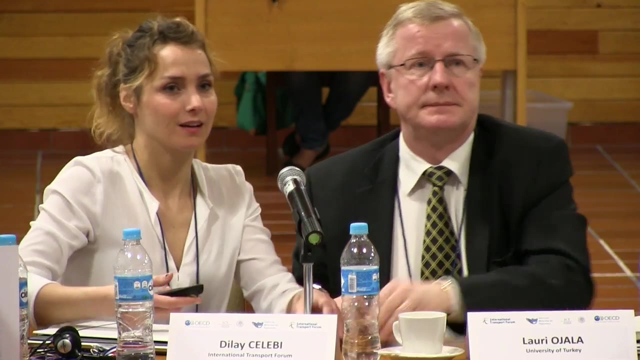 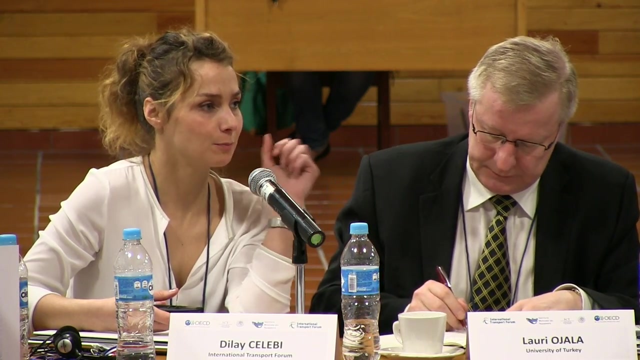 work in towards the policy actions that have been planned and are being implemented in turkey, also understanding the qualitative and quantitative aspects. so should i turn over now to you? yes, as already laurie just said, well, we didn't look at the typical judges, just we didn't make a typical analysis focusing on different transportation modes. but since 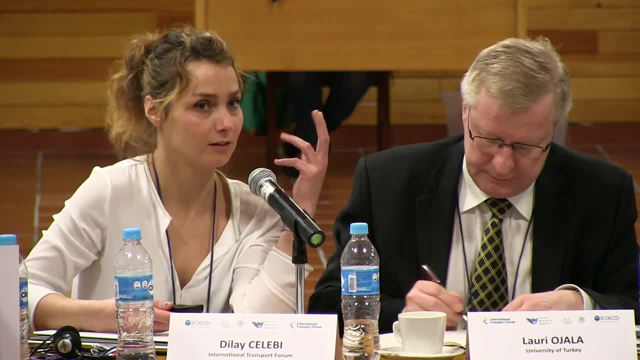 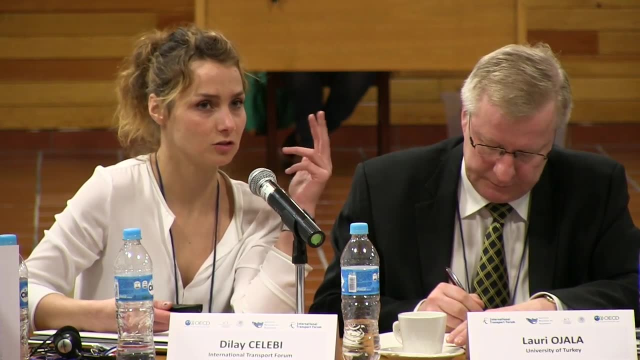 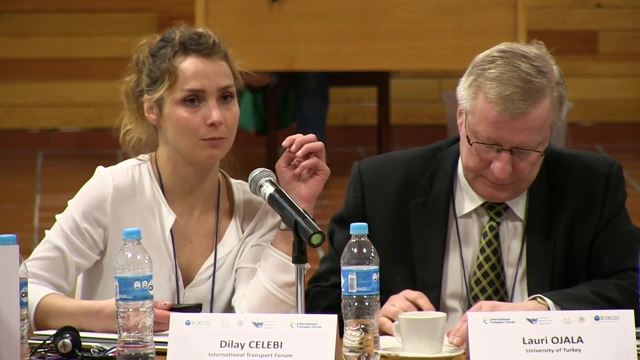 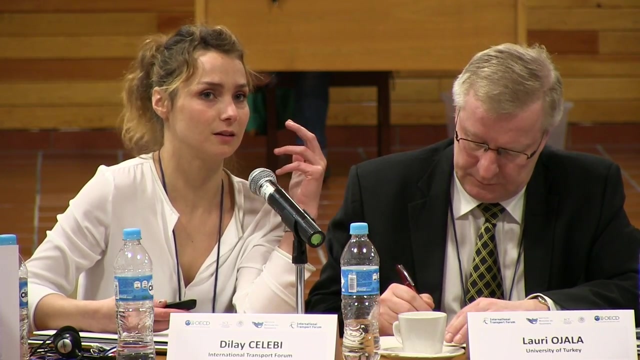 the countries are more concerned about the lpi score and turkey has already put a target score level in the coming years. so we wanted to have a just more holistic understanding of the transportation lpi. just what's going on behind this performance figures, the trend in this performance figures? 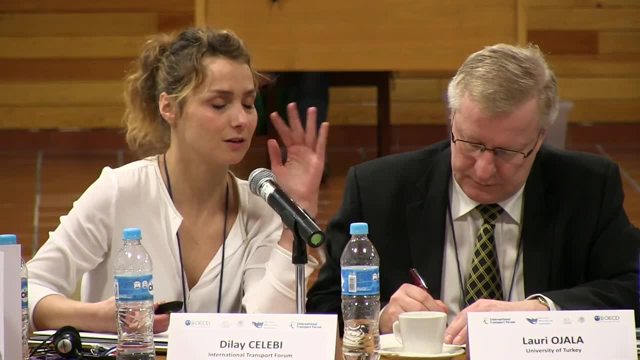 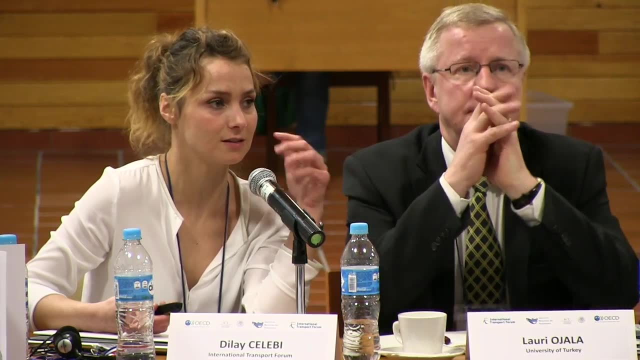 so first of all, for example, we can start: uh, at first i'm just going to summarize our findings. just find more extensive analysis is just uh constraints, i will keep it short. connection is then a different focus. we will keep it short for now because we can come back to the strategies. we managed to stylistic analysis, stability, dynamics and continuity of acreditation along the documents, our data and average data. we will explain what we can get, the priorities for the teams to facilitate between the organization's performance figuresămere andllah, and to figure out how to have a more según obê ve, as we know about the steminationspentoc hoek. compare data, Girl levers, demás pará and I figured it, care lo que habe nos стенh group which, for example, I'm just going to sumarize our findings. here's the paper will summarize our findings. here's the paper. you can just find more extensible analysis. 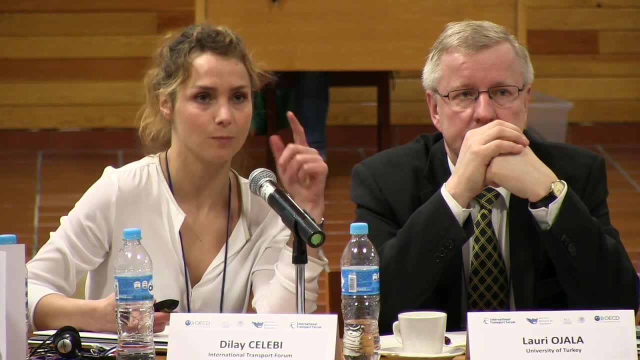 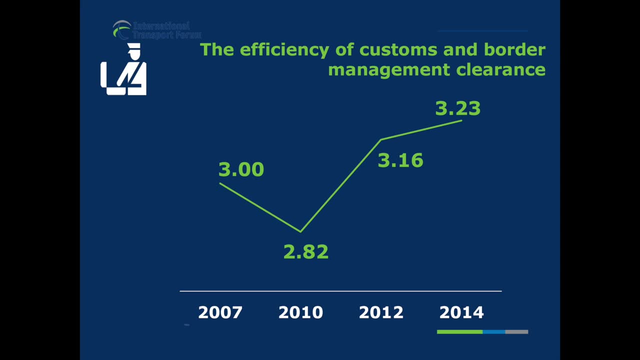 just present you some key findings on these issues. For the customs and border management clearance, you can see that Turkey has improved very well after 2010,. even though it's still one of the two lagging components of Turkey, You can consider as a kind of a basic measure performance measure for the clearance times. 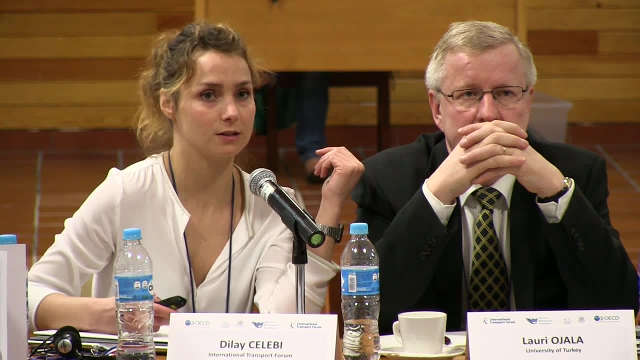 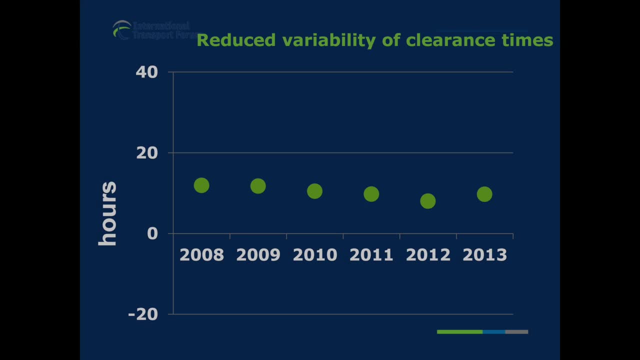 customs clearance times as the average border clearance times, for example. But if you observe in the quantitative measures of Turkey's clearance times, on the average we don't see that much of a change. So the average numbers, even though the average numbers of the clearance times are more or 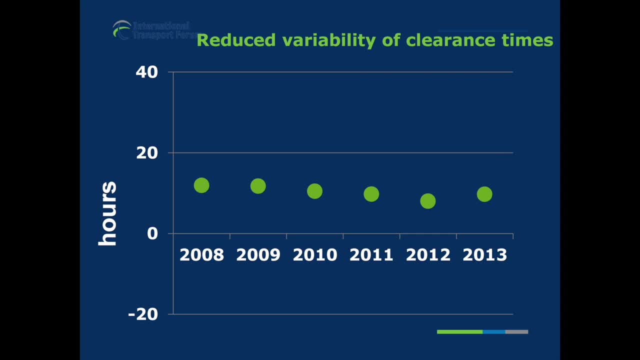 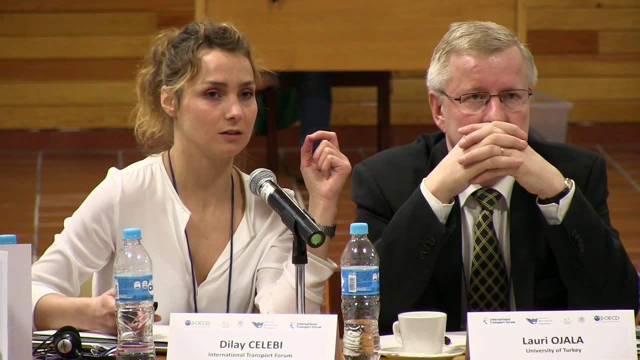 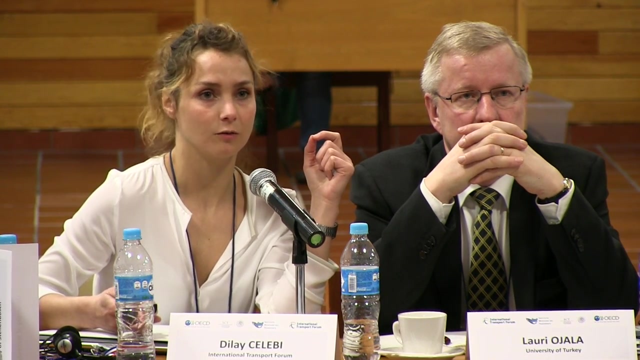 less the same. just you can see that the variability of the clearance times has just decreased tremendously. So this is- I'm going back again- just this: You can see that here in 2000,. after 2010,, there has been a huge increase. 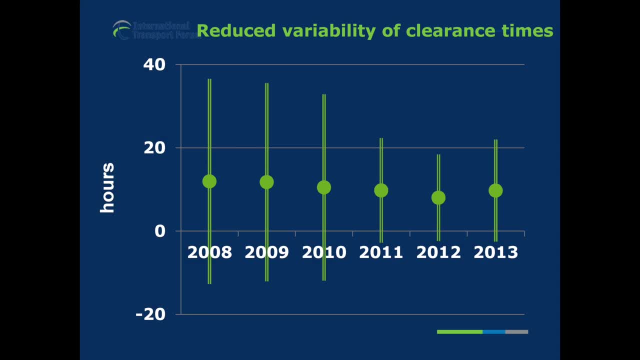 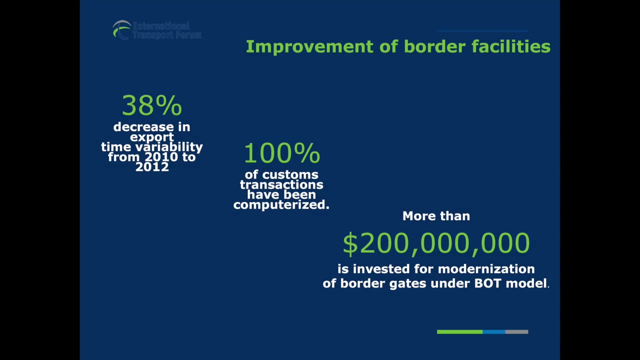 And which might be really related to the decrease in the variability after 2010,. you can observe And how this was managed in the means of policy actions. you can see that just about 100 percent all of the customs transactions has been computerized in this year, in this past couple of years. 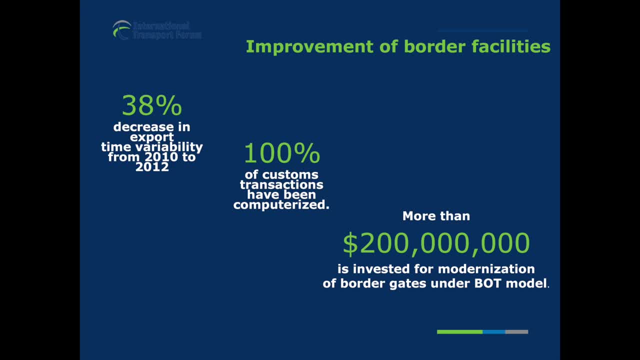 And more and more public-private cooperation models have been implemented. just more than 2,000. billion US dollars have been invested. 200 million US dollars have been invested for modernization of the border gates in 2013.. 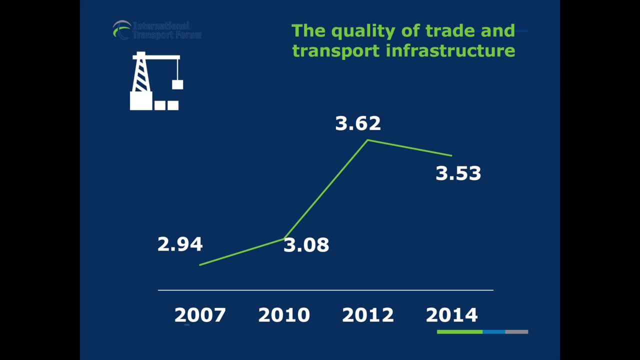 And another measure: if you look at the infrastructure, just the trend of infrastructure, you can see that there is again a significant increase after 2010 to 2012,, but there's a slight decrease in 2014.. So of course, we're just just doesn't direct. 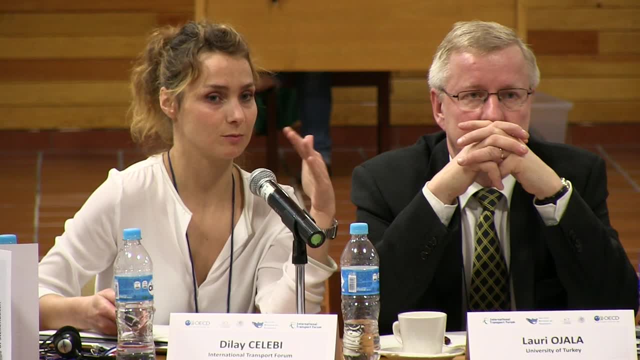 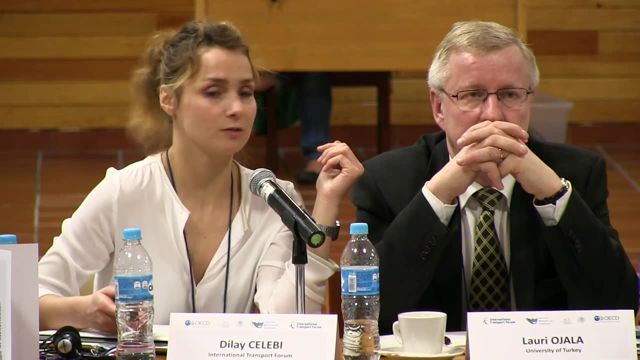 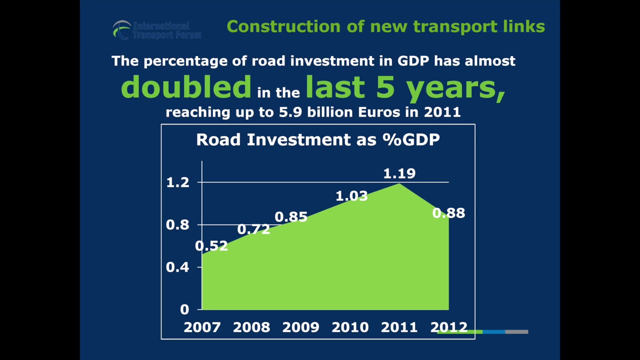 It doesn't directly just show just the investment on the one type of just transportation mode, But by chance or coincidence, you might say. but we find it interesting that well, this figure is actually repeated in this figure which shows the road investment as a percentage. 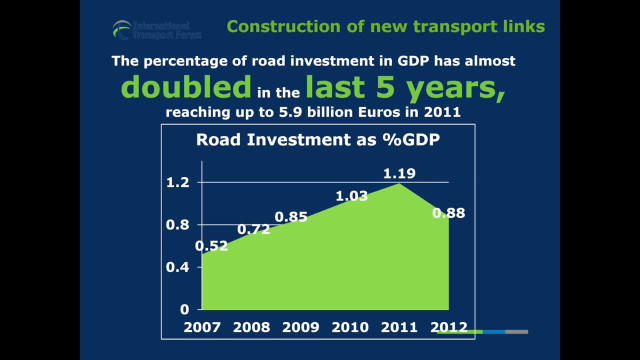 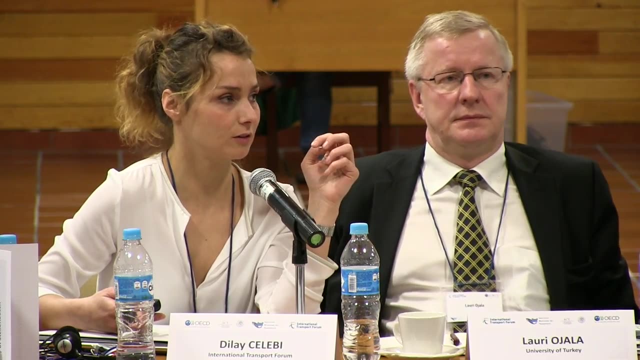 of GDP in Turkey, So the percentage of road investment has been doubled in the last five years. And this is the road- And the road we're talking about is essentially the only road we have seen in the last five years- And, of course, the migration, the transportation of the transport, is the major mode of transportation. 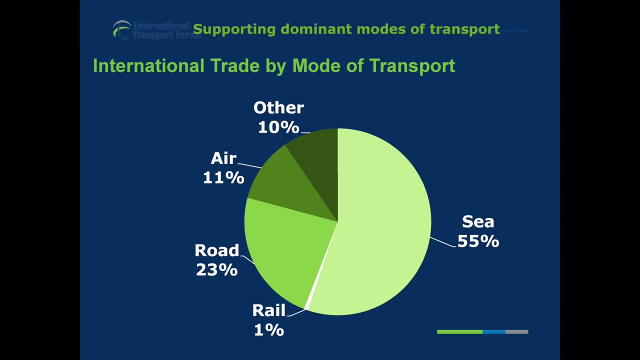 mainly in the domestic shipments, And also it takes a huge share in international shipments as well, much higher than Europe, as you can see in this figure. But of course this has some drawbacks. It is not so just related to-. 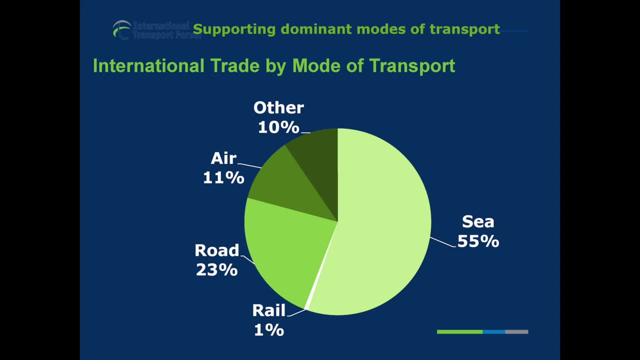 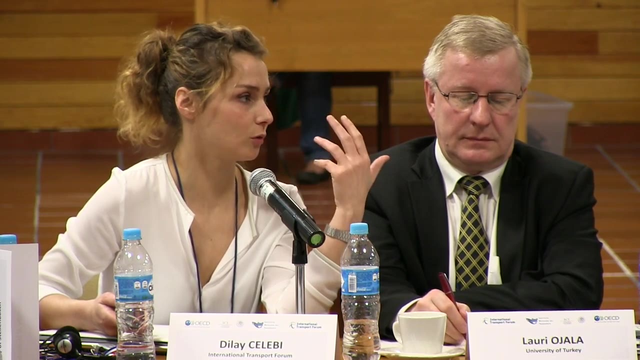 So we see here- sorry before I continue there- as we see here, just the-. this is not a single area, Right, as discussed in the previous session, this is not just the road investment. This is the investment in the major transportation mode. 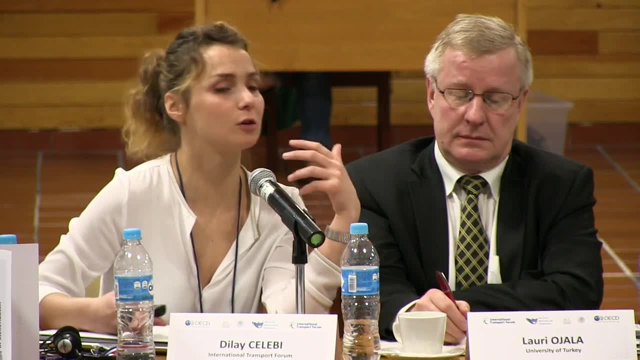 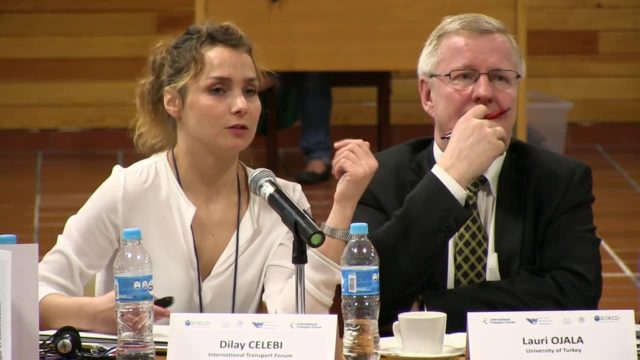 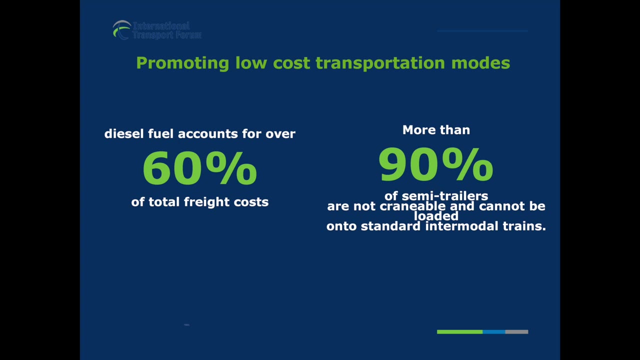 which has been mostly used by the international freight forwarders. So for a different country this might be a different transportation mode as well, And to say that, as a kind of a drawback of this highly dominant road transportation structure, the costs of transportation is very high. 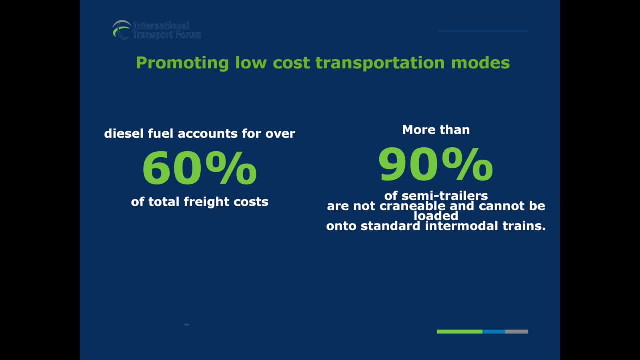 So, according to the study which is done by the logistics body of the International Exporters Association, diesel fuel accounts almost 60% of the total freight costs for the logistics providers in the logistics industry, And more than in terms of the intermodal judges' balance. 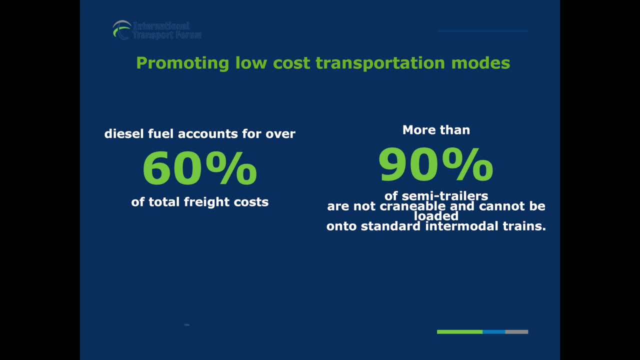 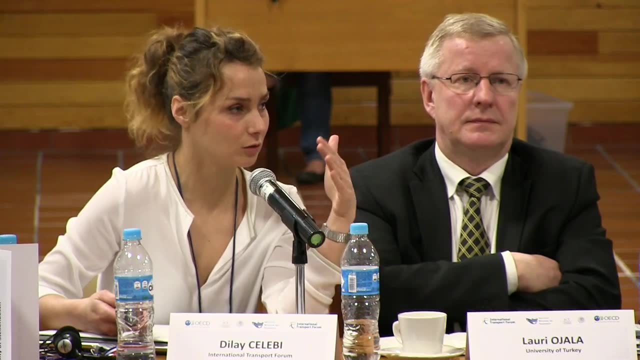 Turkey is below the average, So more than 90% of the semi-trailers are not in Turkey. So it's not trainable to and it cannot be used in intermodal trains. So the connection from road transport to just other modes of transportation. 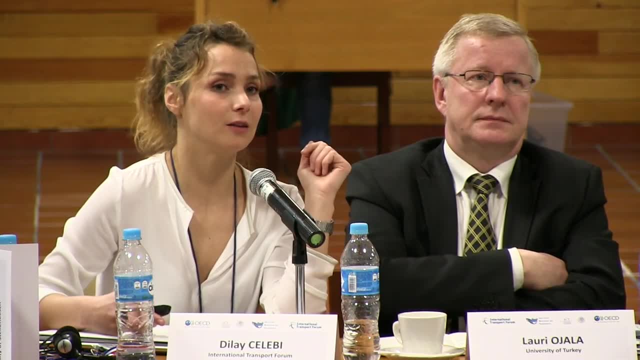 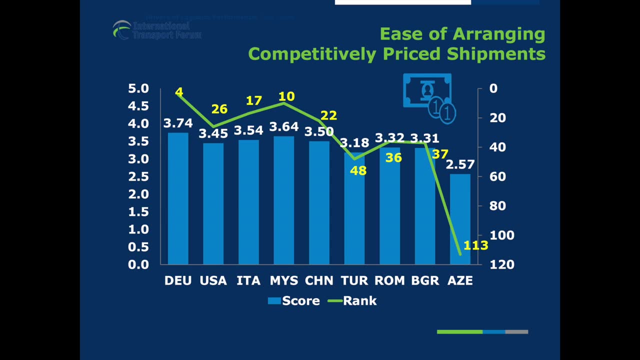 is very difficult in Turkey. As a result of that, you can see immediately on the LPI that Turkey falls below its peer group of countries. So in means of ease of arranging competitively priced shipments, Turkey just lags behind the other, As we can consider, competitive countries in the region. 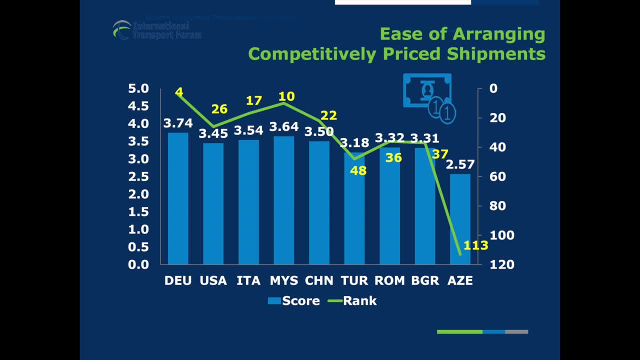 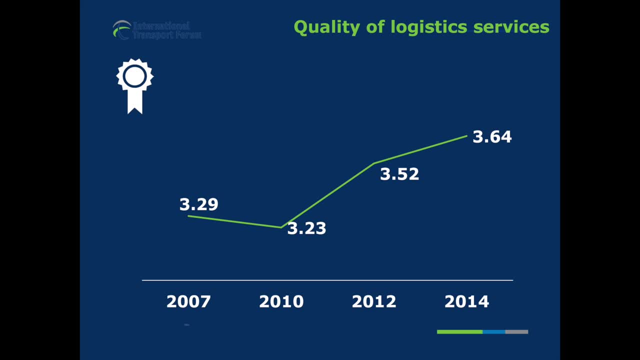 or maybe the benchmarks In terms of quality of logistics services, you can see that there is again an increase in the quality, which is mostly again determined by the strong private sector in Turkey. In the last couple of years, the foreign investment has been increased by incentives. 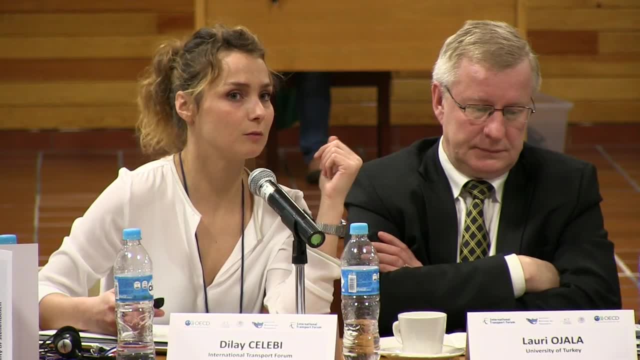 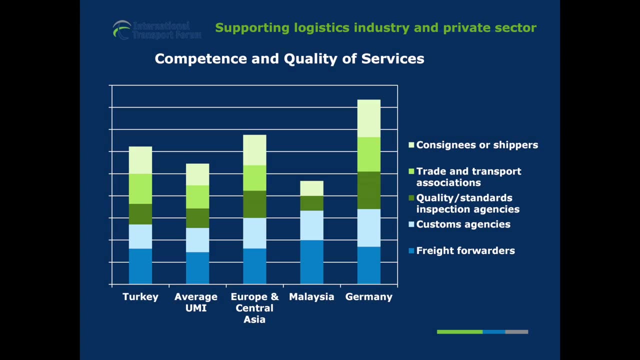 And just lowering the entry barriers in the market. So most of the international players in the market are now started just operating in Turkey, Also the Turkish logistics providers. they got bigger and they started using the economies of scale for increasing their operational efficiency. 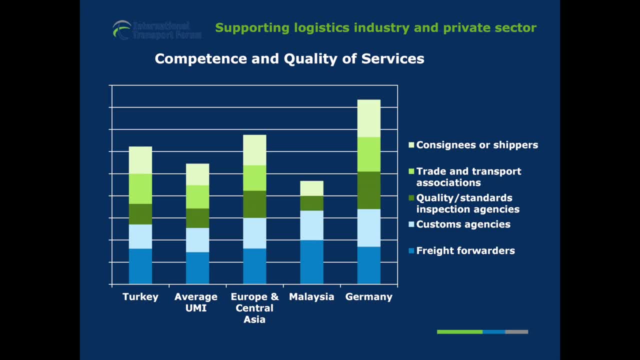 So, as a result, the quality of the services, with the increased competition, has increased. This can be also observed in, again, the domestic logistics performance index indicators. This graphic shows us the competence and quality of logistics services, the percentage of respondents saying high or very high. 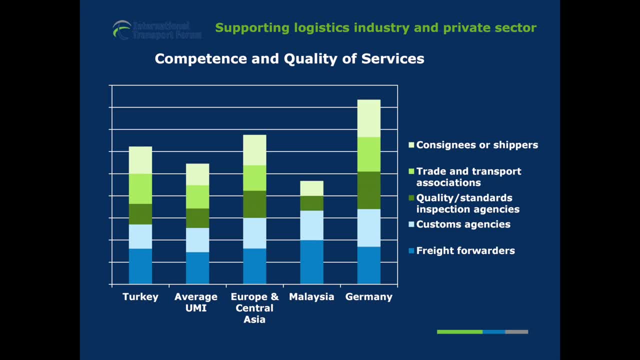 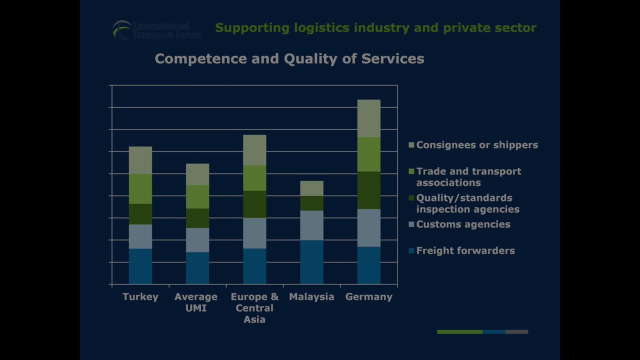 in different terms And you can see that Turkey is even higher, just better than average EMI and even doing better than Malaysia, which is also the top performer in the upper middle income countries And in terms of ability of tracking and tracing consignments. 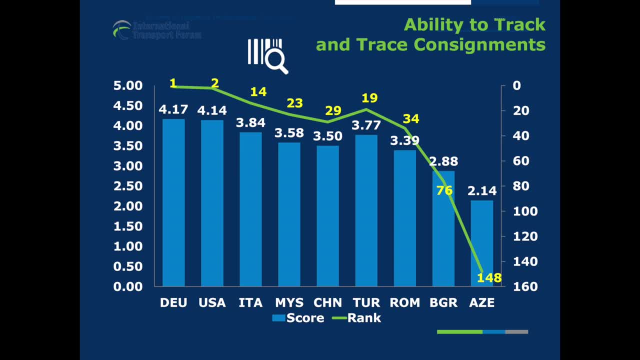 Turkey is again above its peer group and is just performing better than its peer group of countries, And this is mainly related to just the conversion of all this operational activities, logistics activities and just tracking them, and use of computerized systems. 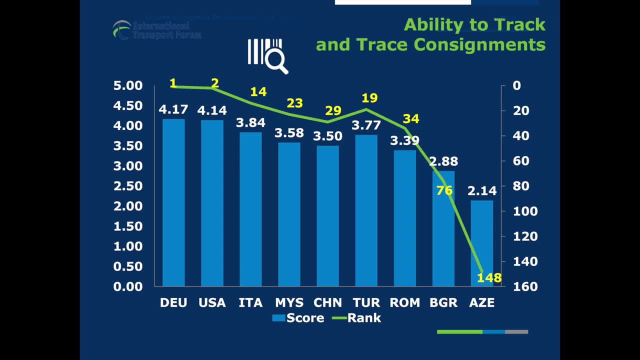 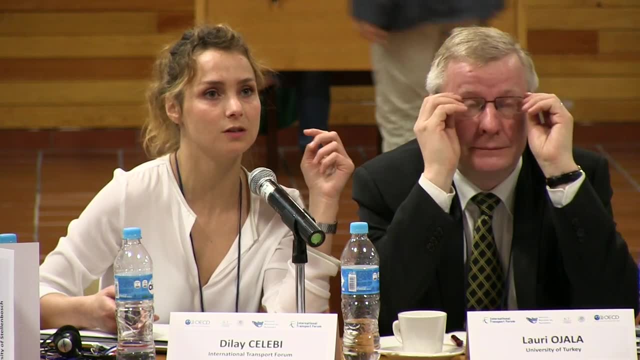 computerized information. So this is a result of our survey just we conducted before we've done all these focus group meetings with the experts. So you can see that most people, just who has taken part, most experts who have taken part in the survey, said that 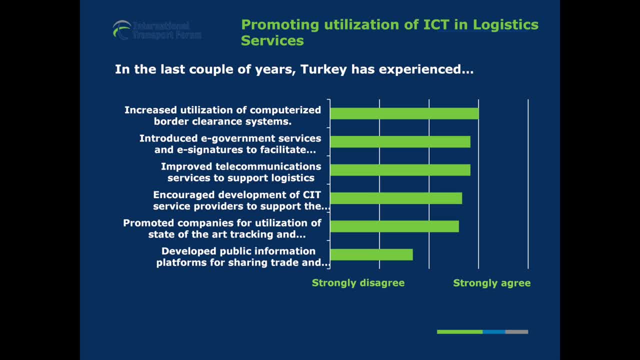 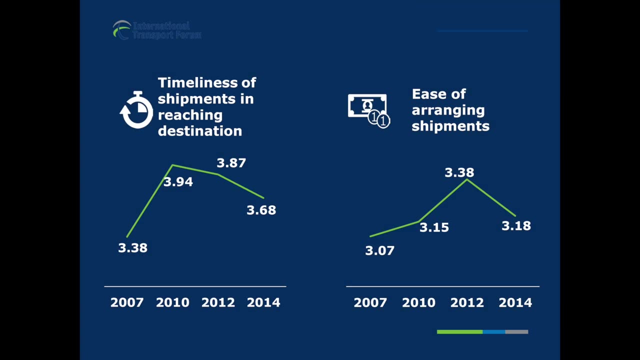 well, in this last two years, there's an increased utilization of computerized border clearance systems or e-governance services, et cetera. And finally, just I would like to show you just two just declining trends, which is in the timelines of shipments. 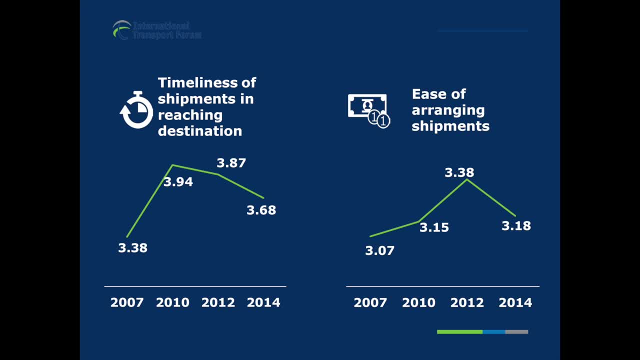 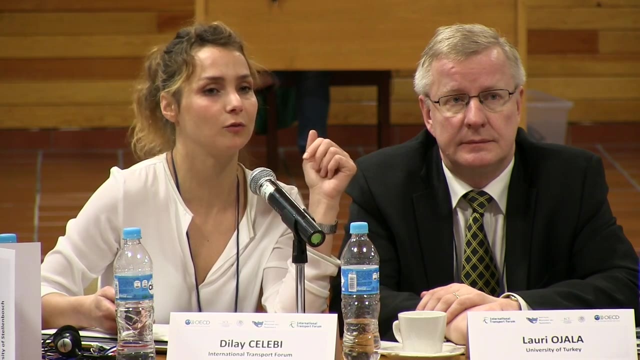 and ease of arranging shipments, which is the price, and the timelines, which more or less, you can see that are correlated because of this delay which might happen in the borders. So last year, after 2012,. between 2012 and 14,. 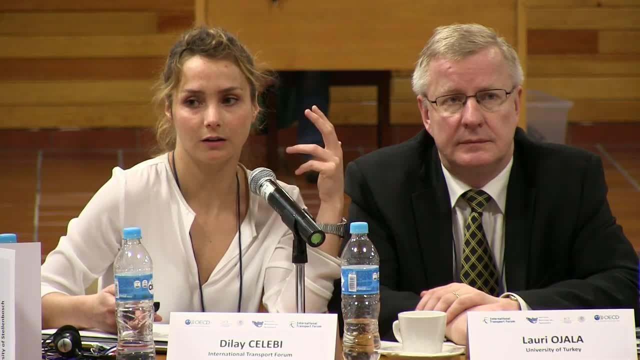 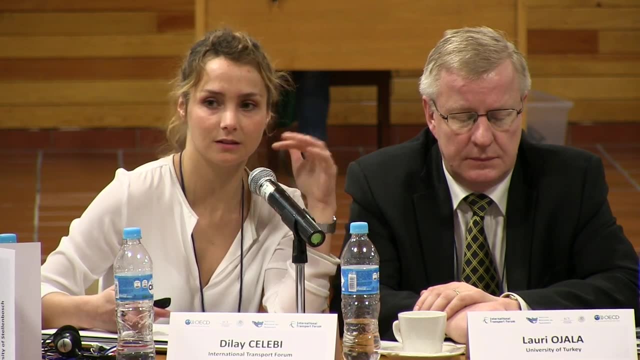 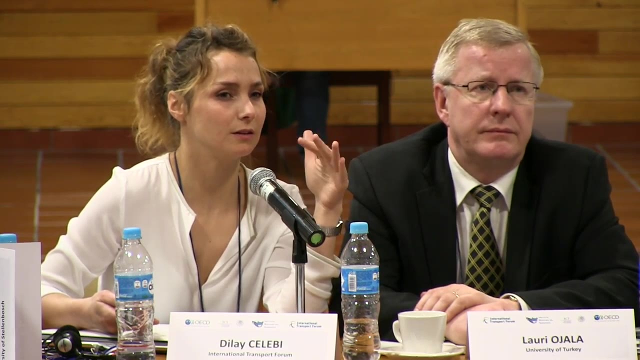 you might have heard about all these political conflicts around Turkey, The war in Syria and the Middle East, the political disputes in the Middle East. So for some time after, in the late 2013,, the Syrian border was completely closed, for example. 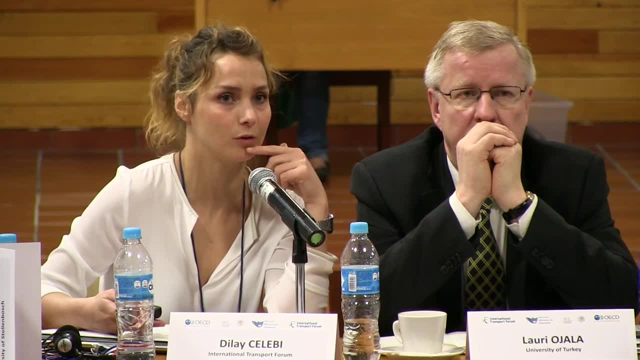 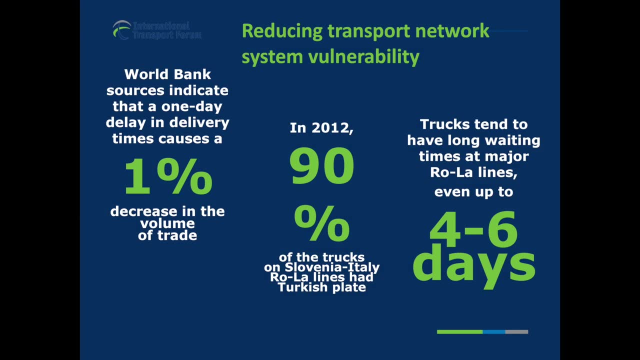 which has stopped all the traffic, all the trade traffic, in that border. And also there have been some political conflict with the European border with Bulgaria and Romania. so which has you just converted the Turkish companies to look for alternative roads for reaching Europe? 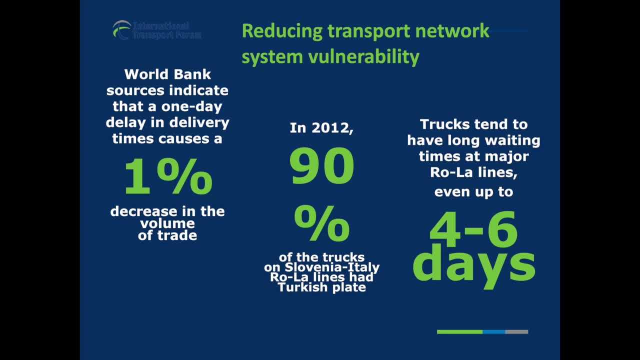 And then because of the kind of congestion on these roads that there have been, the Turkish trucks tend to have long waiting times, which might even go up to four or six days just waiting for the roller lines. Just as a clarification, this roll-up line: 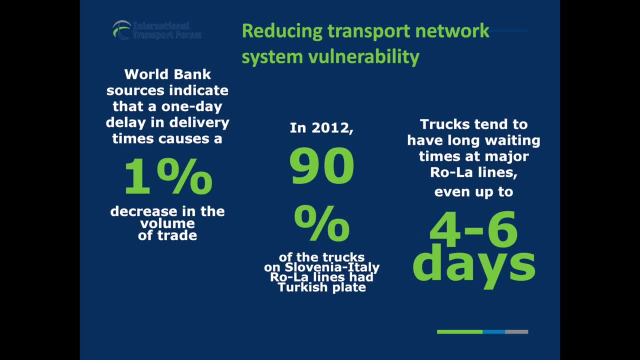 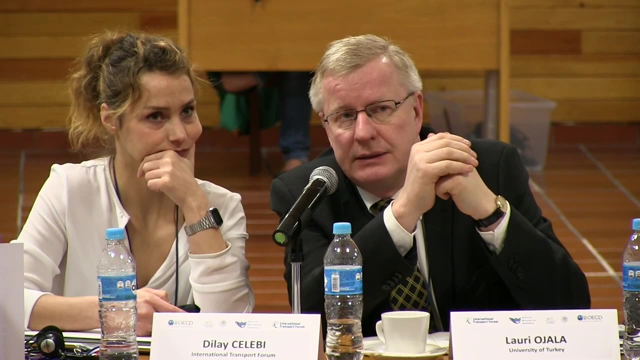 is a specific term for coming from the German words Rollerlandstrasse, meaning it's a just piggyback- trucks or trailers on rail, especially through Austria, typically on the Slovenia-Italian connections or through Austria. So this is what it means. 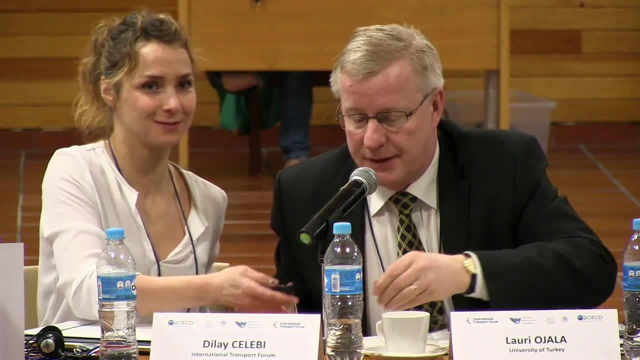 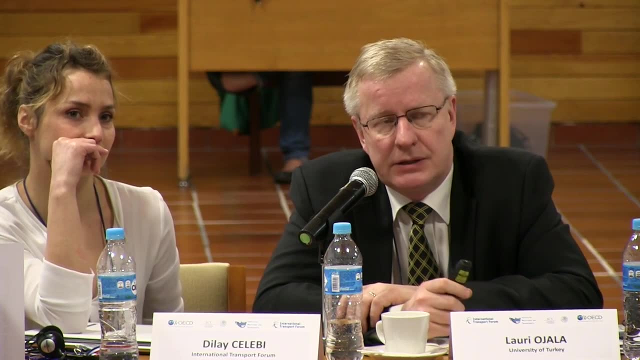 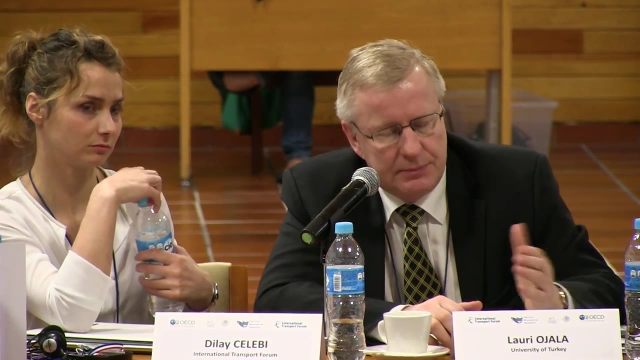 Yes, I actually finished, Laurie, you can continue. Thank you. So there are some issues, of course, of regional or local character, but the exercise was actually. the purpose of this exercise was to take the LPI findings as a starting point. 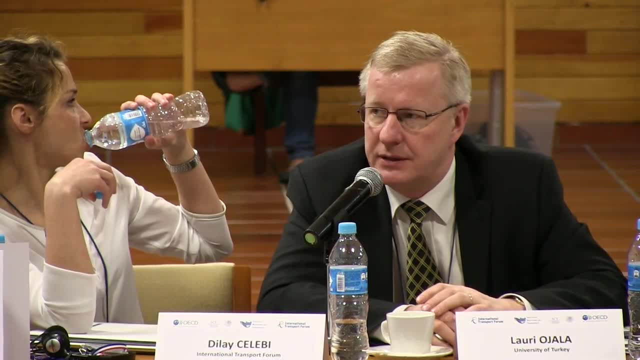 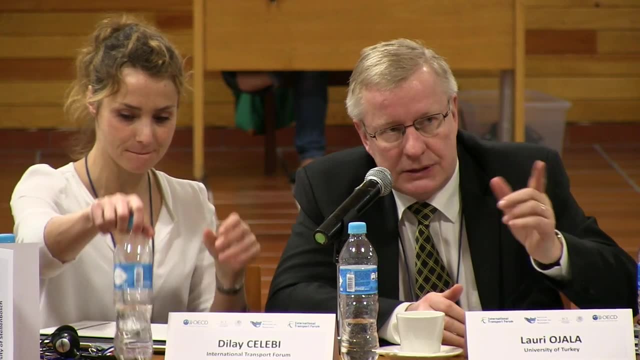 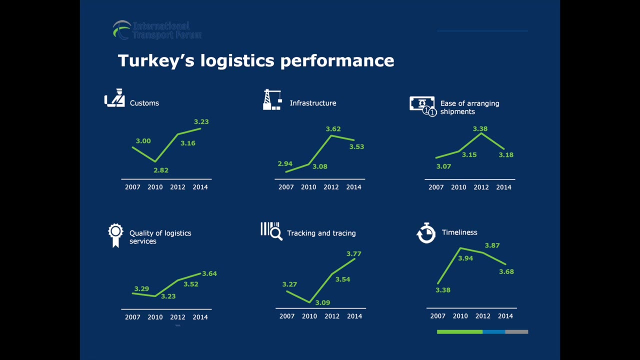 and to understand better what lies behind these figures. That's why we also call this exercise Behind the LPI on Turkey. Just coming back to those scores and numerical indicators, each one of those six dimensions actually was rated in a score, from one, the lowest, to five. 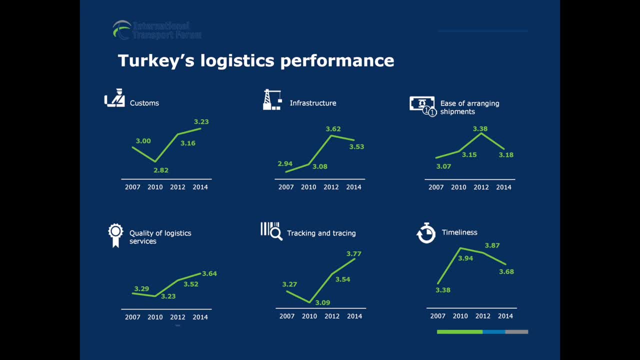 which is the maximum. so if you are somewhere at 3.9, or 3.4,, you are already at relatively high score levels. And an additional thing that I would like to add is that when we use these, I'm saying we- 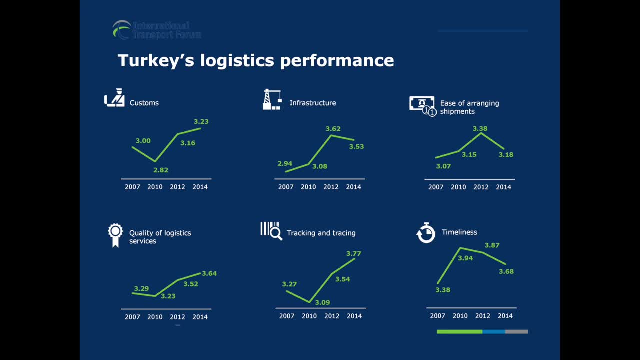 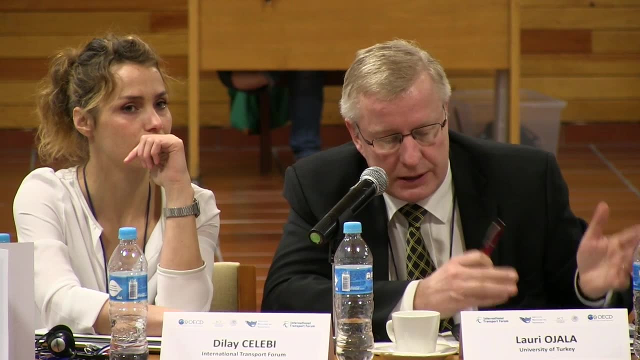 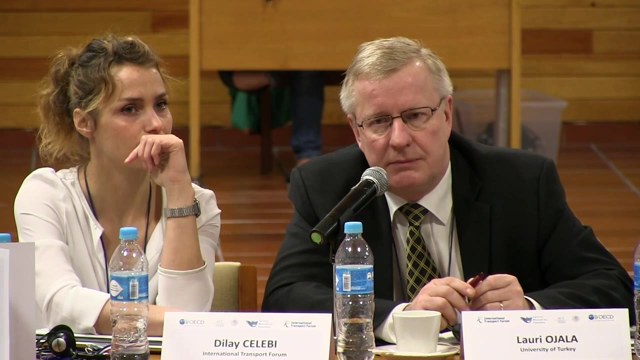 because I'm one of the co-authors of this LPI report, as many of you might know. when, for example, Turkey or Finland, or Mexico or Germany is evaluated and compared in these international ratings, all these ratings come from, for instance, 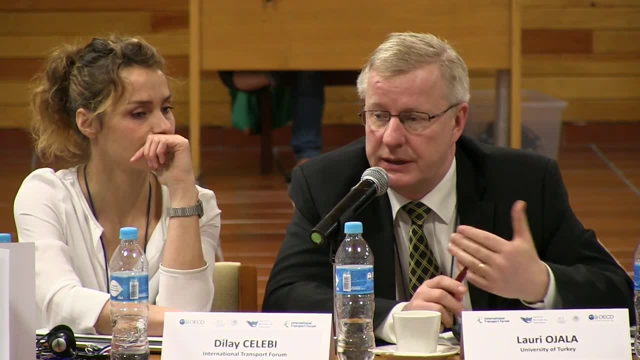 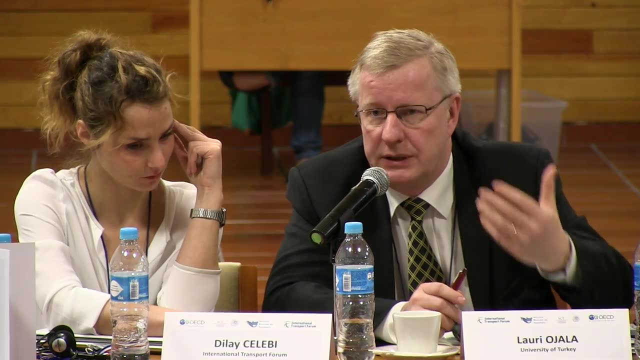 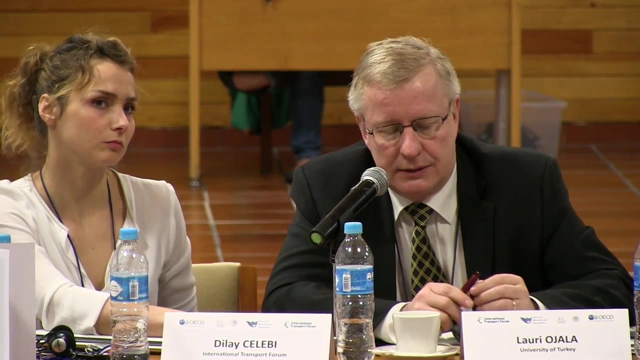 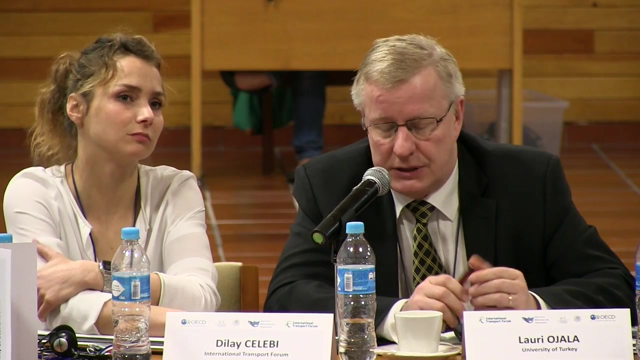 outside that particular country. So the respondents who are rating Germany or Mexico or Turkey are from outside that country. It is also important to realize that this is more like an external freight forwarding, specialist professionals aggregate perception that is condensed into these figures rather than being just the Turkish respondents rating Turkey which we have on the 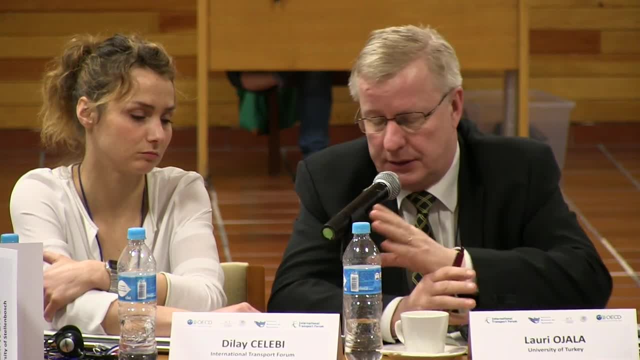 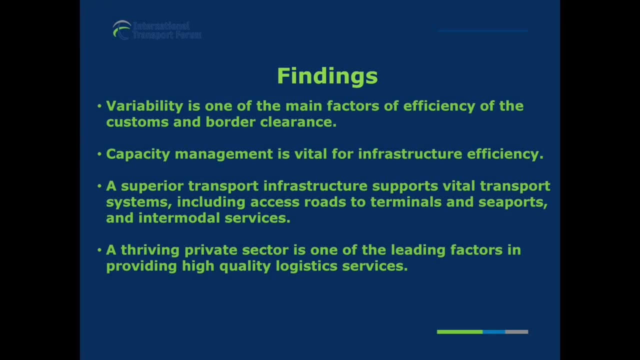 domestic side on some more numerical. but this international comparison is coming from outside, Coming back to the findings we had here. so typically on the border crossing activities, reducing the variability of waiting times or clearance times is a global issue and internationally documented that it is one of the important aspects to make. 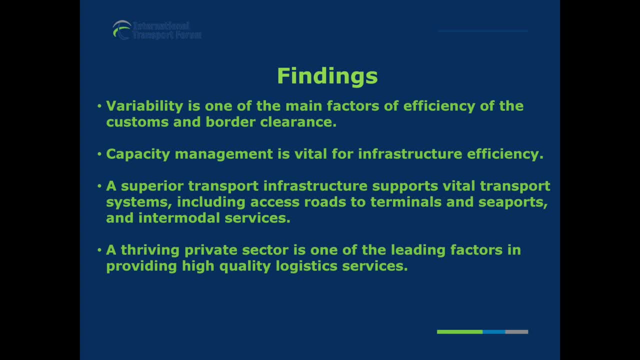 transport more efficient, More predictable, and I think it was also in Alan's paper that underlined the knock-on effects or the bullwhip effects or in different ways. so if you have a lot of uncertainty at one stage or one node of supply chains, it easily and 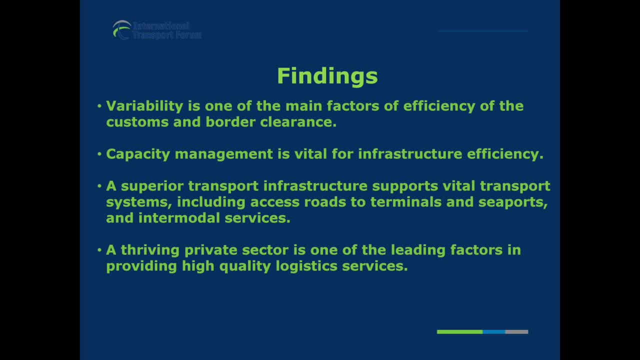 typically multiplies in the way that you, for example, traders and companies, have to keep much higher inventories to be able to cope with the situations and in that way the inventory running costs and all related costs may be multiplied. and I'm not referring to this whisky type of production in Scotland here, but 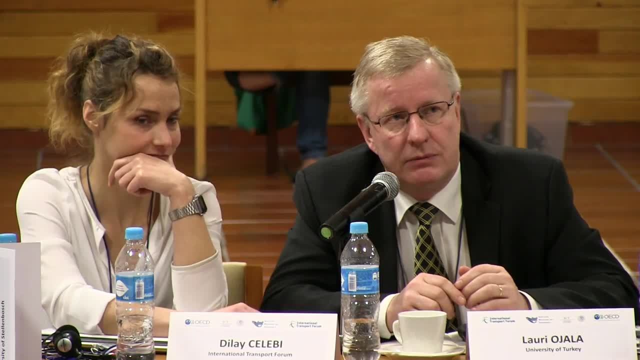 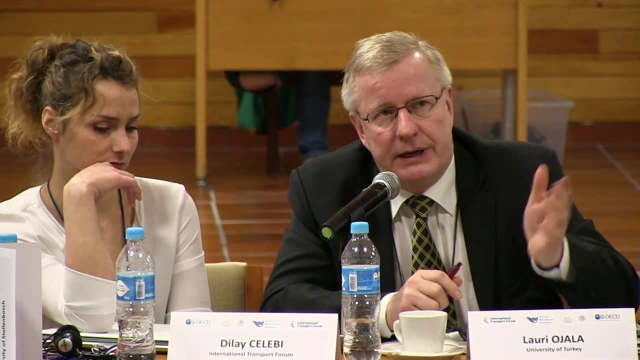 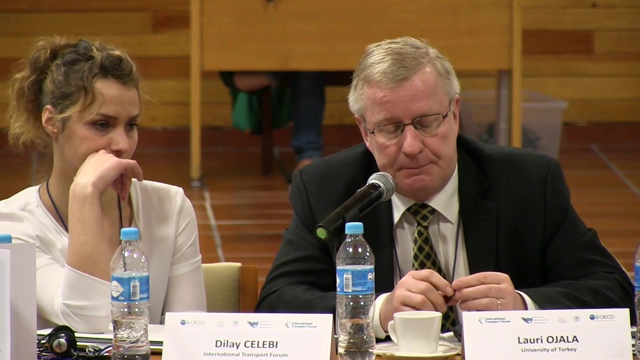 generally speaking, this is a big issue and I think this is something where Turkey has been quite successful in reducing this variability in border crossings. Another finding, which is more general to the LPI as well, but has some bearing to Turkey as well, is that when we talk about customs and customs clearance, 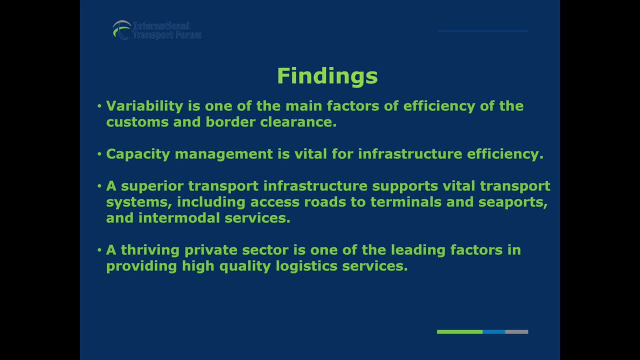 it is very often not the customs administration as such which is the main culprit or the main bottleneck. it is very often the other border agencies, be they veterinary or phytosanitary or some standardization agencies, and, in particular, it is the cooperation between 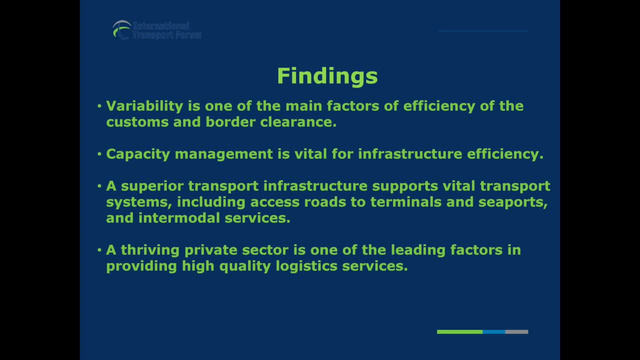 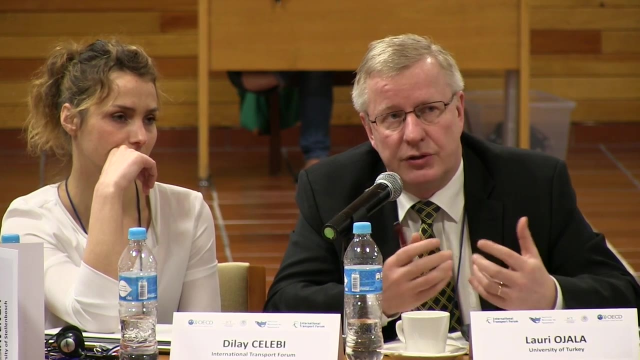 these different agencies. that is often key. This is very much the picture in much large part of Latin America, if we have understood it correctly. This is very much the picture in Africa, parts of Europe, Asia as well. So the interagency cooperation is also vital from the policy making point of view. 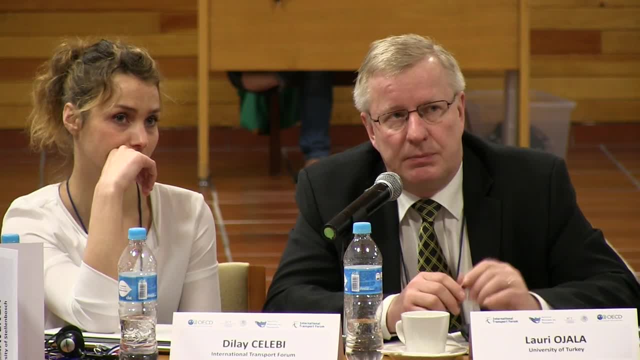 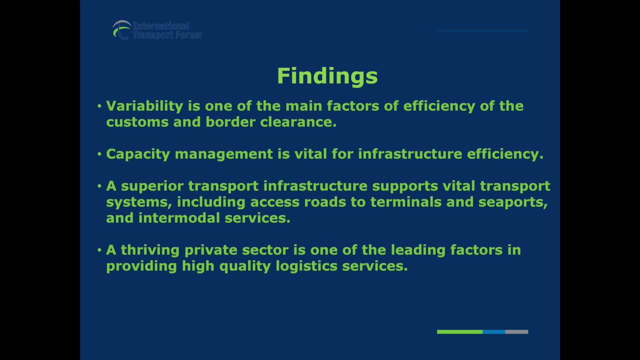 Also understanding the second bullet point here, the capacity management, meaning that especially for those nodes in the transport network that can create bottlenecks due to service issues, like border crossing points, where you have a service element in passing through, it is also important to understand what sort of investments 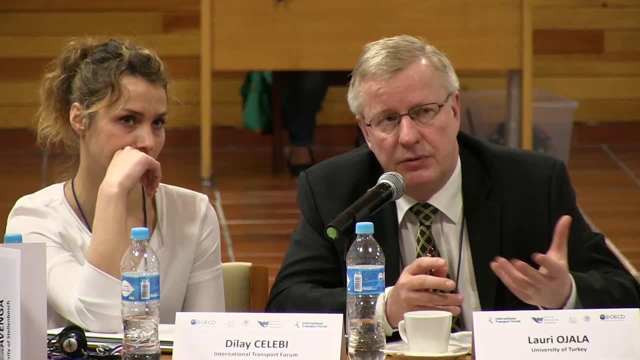 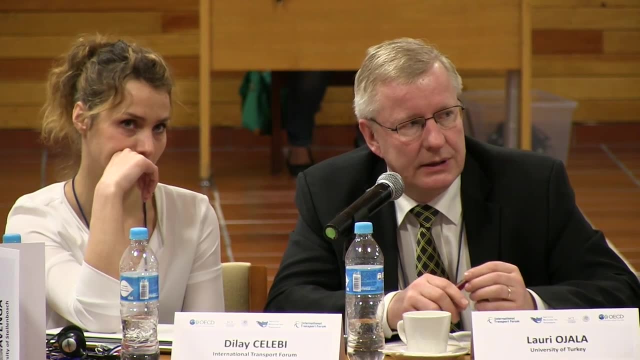 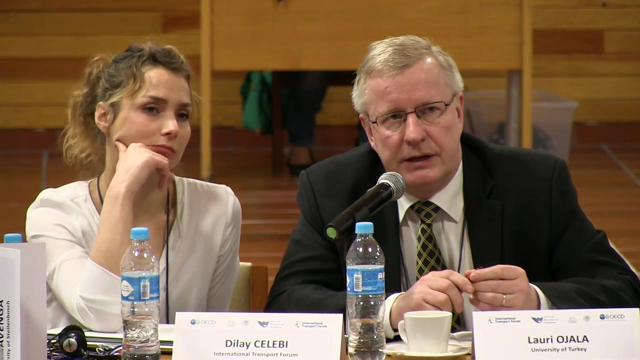 do you really need to cope with the normal flow of passengers on one side and cargo on the other? and how can you cope with the peak moments, be that within a week, within the month period of the year, or so forth? Of course, if everybody builds every infrastructure for the peak demand. 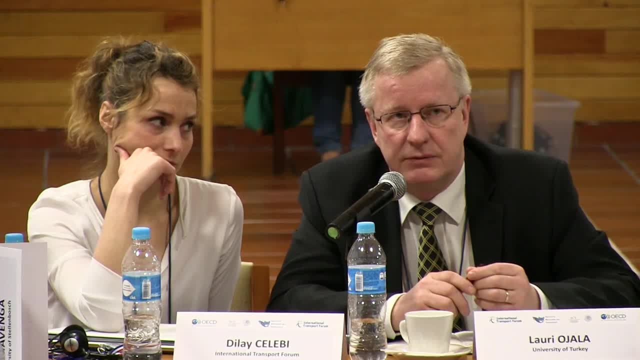 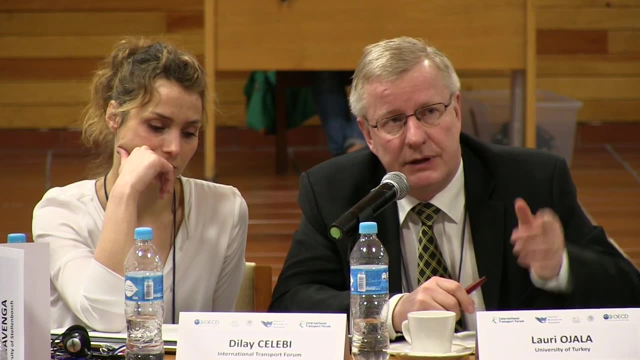 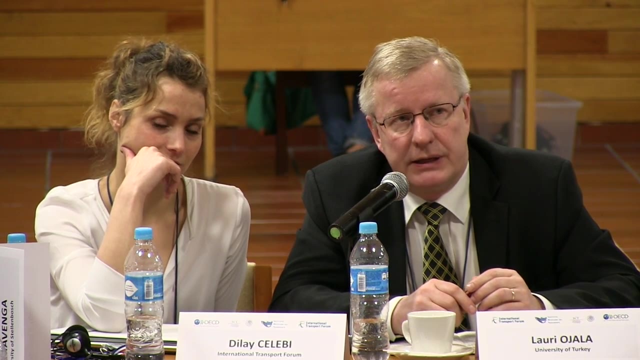 it will be extremely expensive, and this is, of course, not what is meant by this, but, to understand it better, how to dimension the infrastructure needs to the fluctuation and also the top of demand. It also came very strongly from the findings that 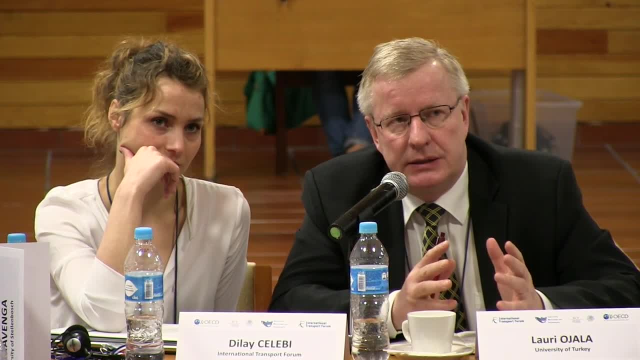 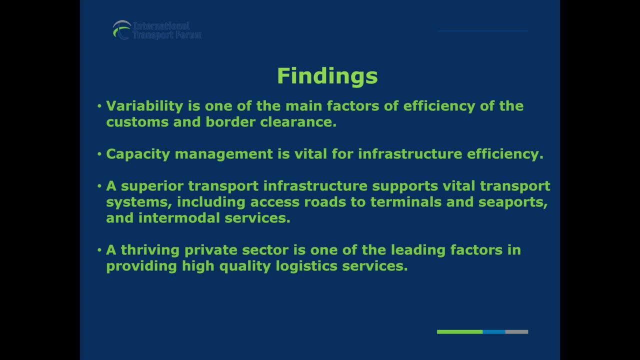 once you create and establish and maintain also good transport infrastructure, it is a platform and the basis on which you can then have a reliable, high-quality services. But of course transport infrastructure in many cases is just the necessary condition to have a well-performing logistics, but it is not the defining condition of doing so. 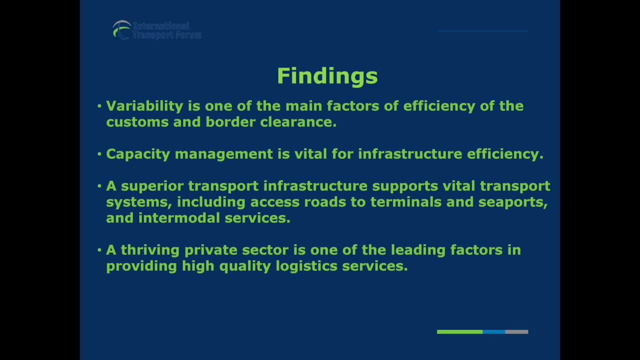 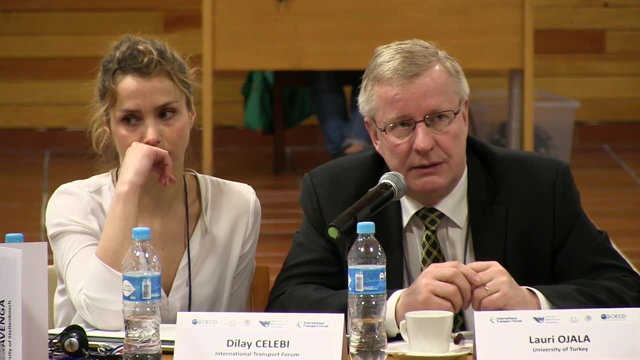 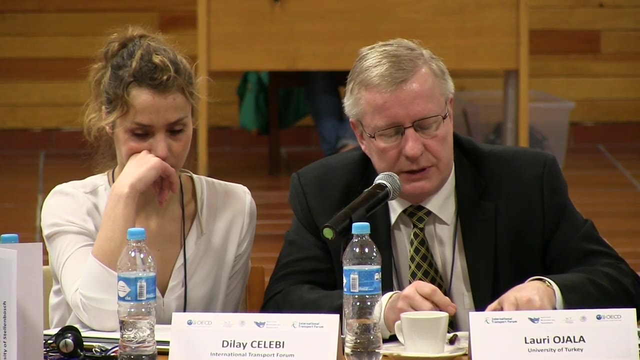 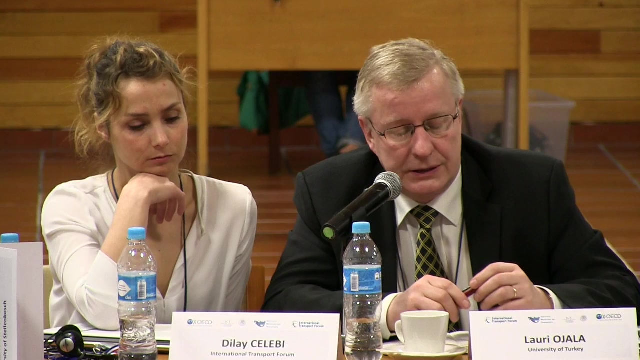 And, as was mentioned in one of the comments in the early morning, countries at different stages of development have different needs in terms of basic transport infrastructure to get it, and then moving forward to more advanced business environments where the service offerings become more important If you are in a high-income country. 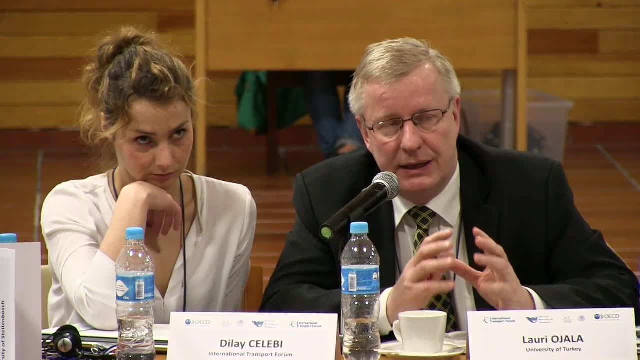 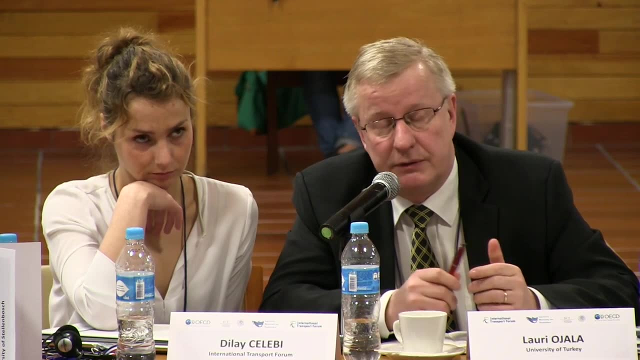 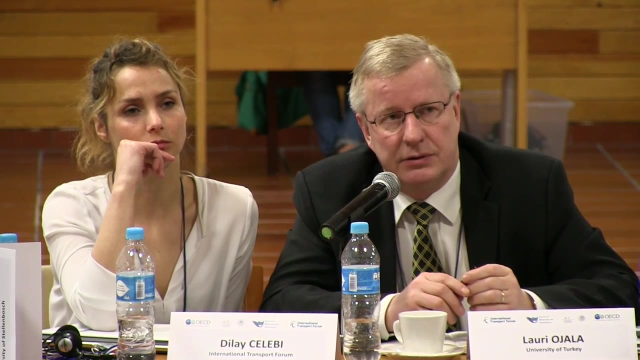 infrastructure typically already, to a great extent, is there, but how do you provide the services on top of that? infrastructure becomes much more, relatively speaking, much more important than building an additional road link between two places or additional expansion of a particular terminal. 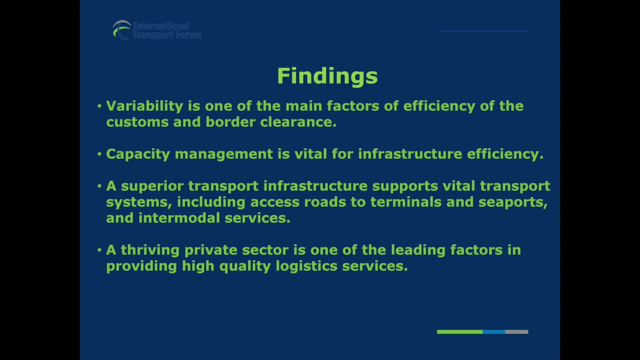 Finally, it was very clearly seen in Turkey that the private sector, both in manufacturing and trading businesses and also in the private sector in providing logistic services, has developed tremendously over the past 10 years. In the last 15 years in Turkey we also saw the very high increase of Turkish exports. 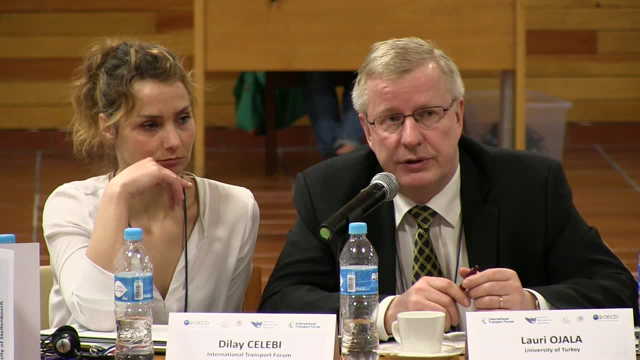 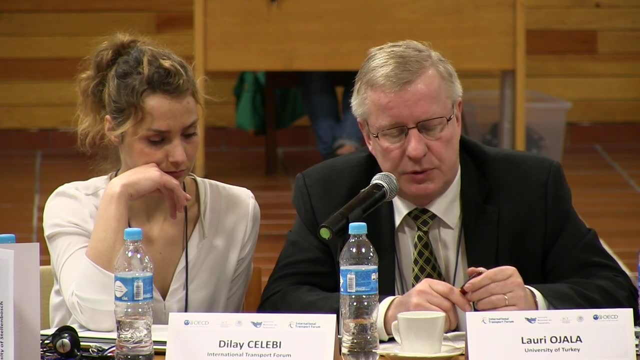 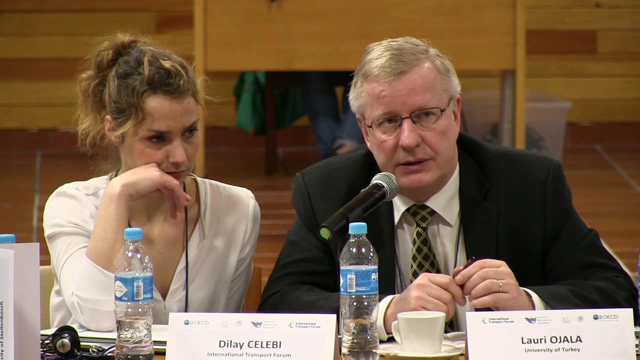 starting from around 2001 and 2002, when the agreement with the European Union was signed, which was one of the big boosters of Turkish exports and also economic growth. as such, The private sector is a thriving private sector is one of the key factors in providing also high-quality logistic services. 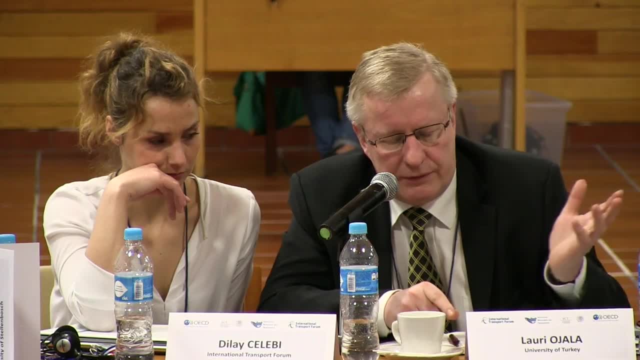 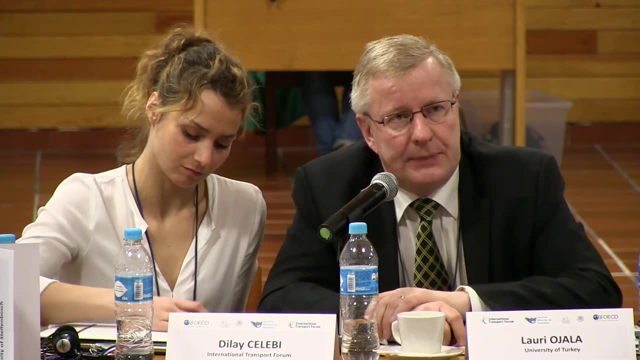 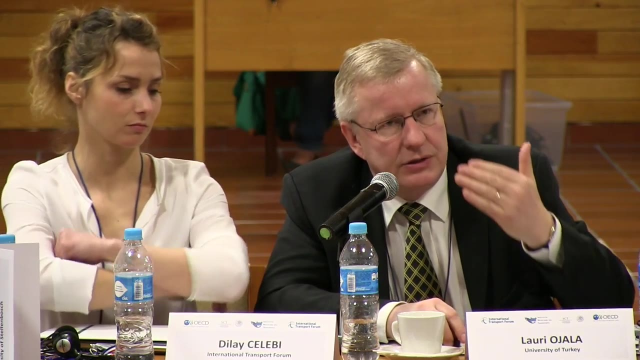 coming slightly back to what Jan was also referring to with this chicken and egg problem, in a way which one comes first. I mean Turkey is also a case where this very rapid economic growth and in particular rapid export growth has also mandated that the logistic sector has had to develop very quickly. 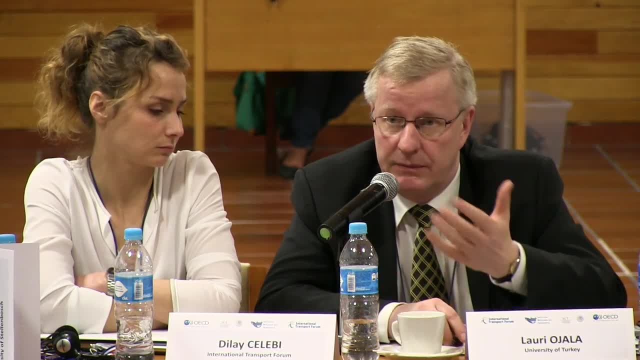 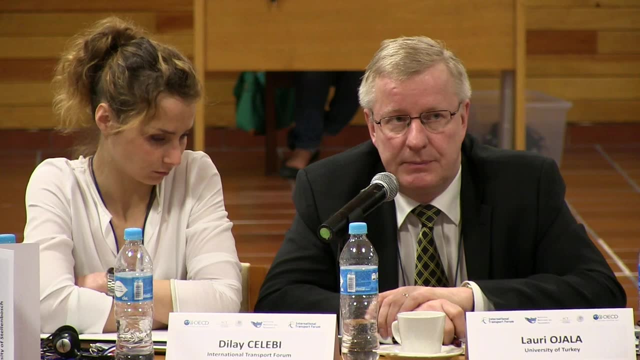 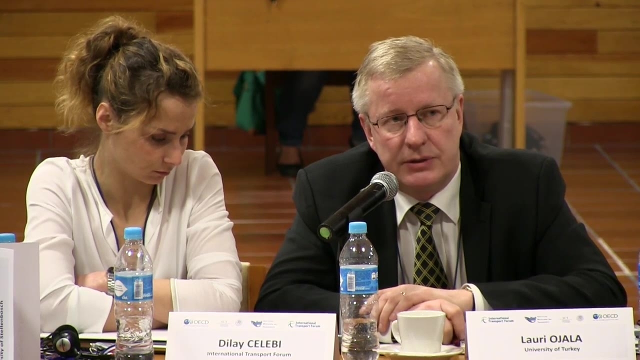 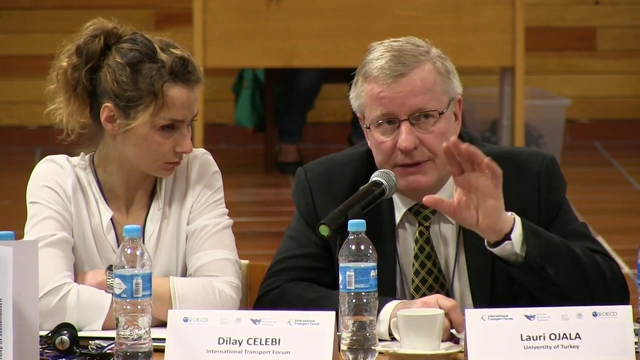 both through foreign direct investment companies from outside Turkey establishing their activities, but also domestic companies being able to quite quickly come up with the situation and start to provide services that are high quality, good sort of a good quality price-quality ratio services. But having this is really one of the key things.